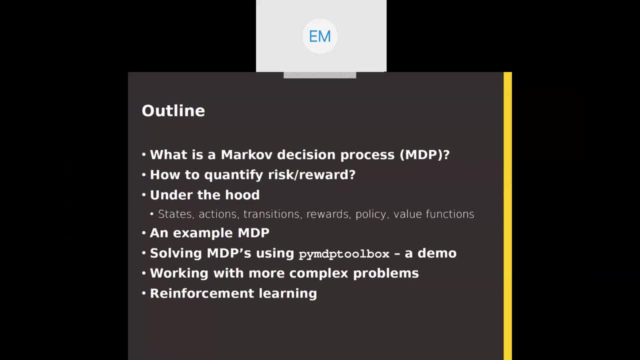 And then that might be kind of theoretical. so we're going to go through like a concrete example of an MDP and that will involve using this PI MDP toolbox package, which is like a Python package that somebody- not me- wrote to solve, like simple versions of these types of problems and reinforcement mining, which is the combination of machine learning and MDP. 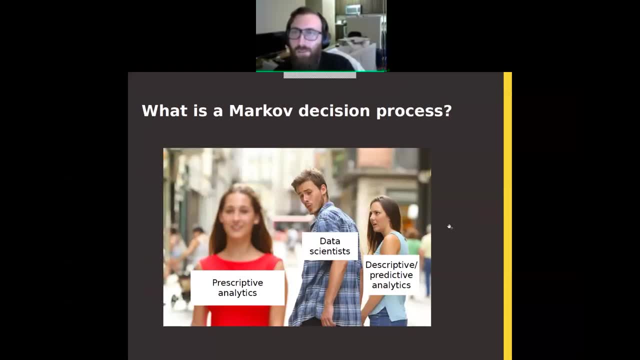 So what is a Markov decision process? So I like to bucket analytics into like three different elements, which I guess would be descriptive analytics, which is where you're kind of looking into the past and summarizing or finding patterns of what happened in the past. 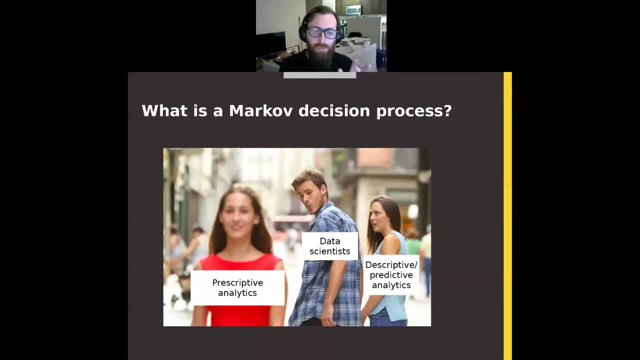 There is predictive analytics, which tries to use the past to forecast the future, And then there is prescriptive. And then there is prescriptive analytics, which is where you say: I want to be somewhere at this point in the future. How do I get there? 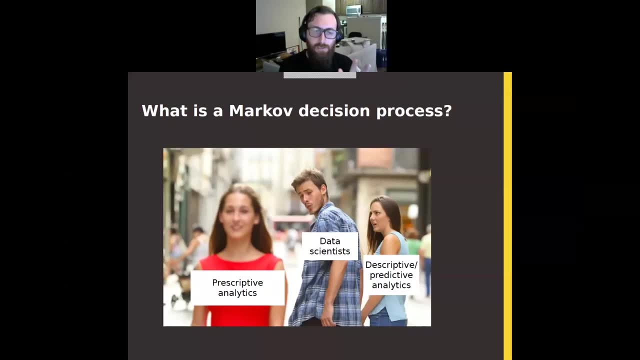 Prescriptive analytics will tell you how to get there. So MDPs kind of combine all three of these aspects together. Based on where you have been and where you want to be, they will tell you how to get there and what sort of. 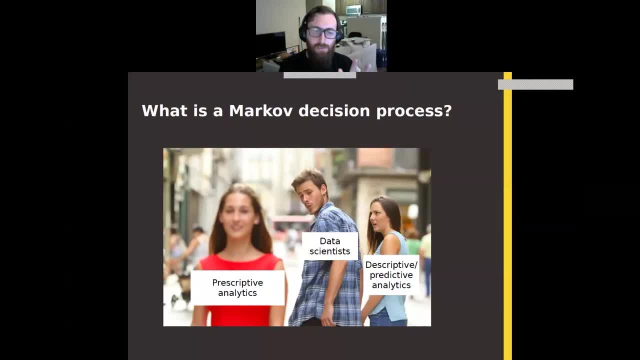 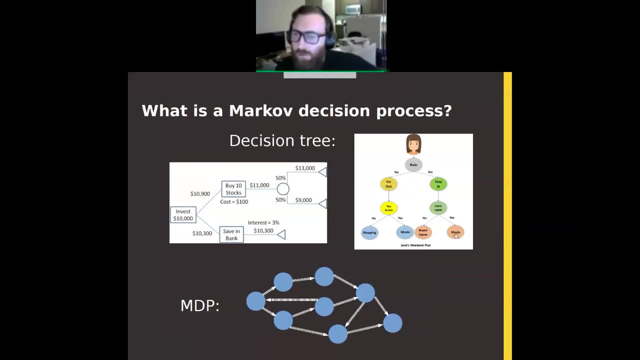 goals you'll work towards. you'll pick up along the way. Yes, So you might already be familiar with like a kind of a more simplified version of like a full MDP, which is a decision tree. And so decision tree, the way that works is you start off somewhere. we call this the root node. 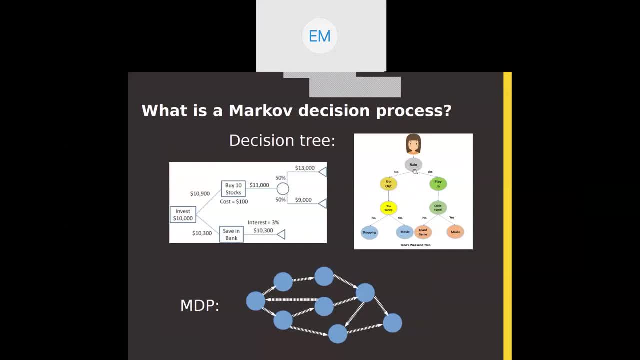 And at the root node, you're presented with various. And so, at the root node, you're presented with various, And so, at the root node, you're presented with various options for actions that you need to take. I'll just go with the example on 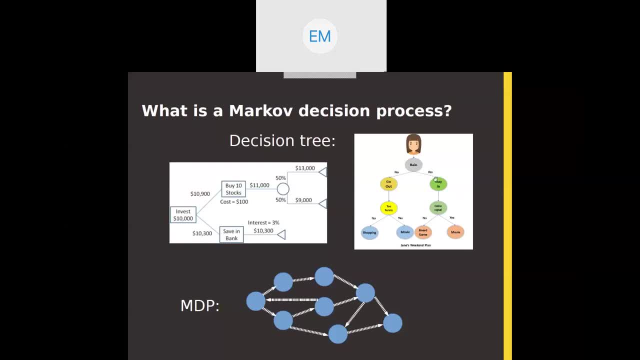 the right. so, like it's raining out, do you go outside or do you stay in, yes or no? and based on that decision, then you either take one branch or the other, and then you go down and you're presented with another, presented with another option for an action to take and make it just another decision there, and so on. 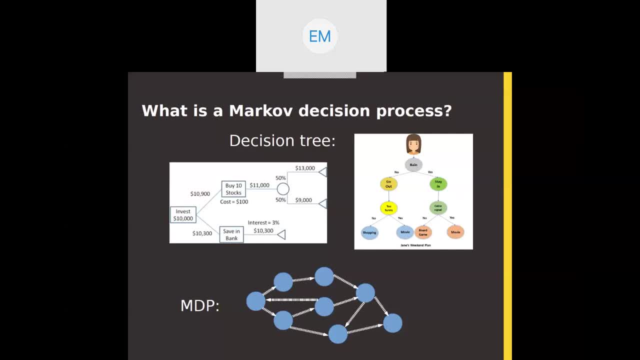 and so forth. so you kind of like continue down this, this tree, until you reach your terminal state, final state, which is the place that you want it to be, hopefully. so trees are actually like a special case of more general graph which can, which is basically just a linkage between nodes, and so you can see. 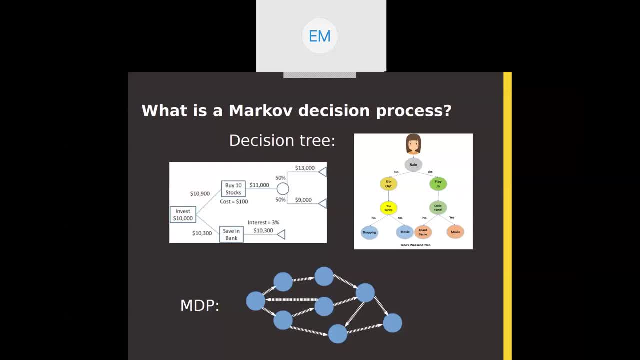 the tree is always the root node, which is kind of special, and it branches out from the root node. with more general graph you could have between any one node with any other and potential transitions, and so an MDP kind of operates in this more general general sphere rather than a simplified version. 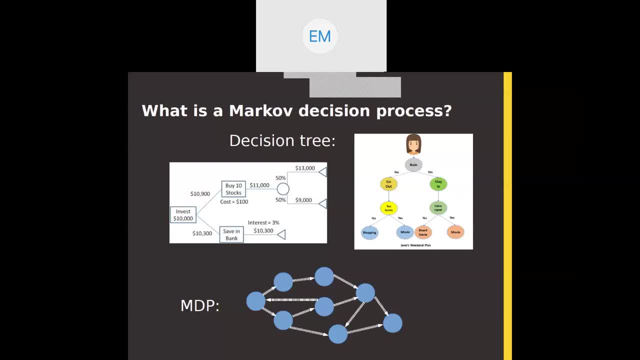 and this allows really complicated behavior in your decision making processes like loops, for example. you can start off in a certain certain node and by making a sequence of actions and decisions, you can eventually end up in the same state that you started at, or maybe you could visit it multiple times. it can get complicated, but it's also very flexible. 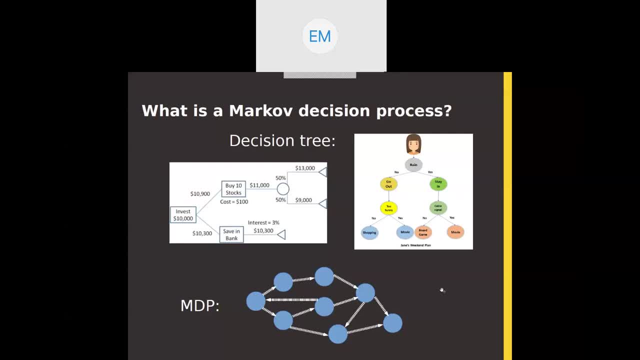 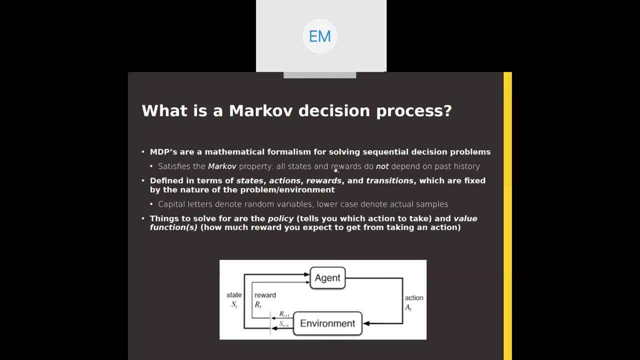 and generalizable and useful. all right. so what is it more? formally, it's a mathematical framework for solving sequential decision problems. by sequential, I mean, you don't just like, you don't just choose at one point do I take action A or action B, and then that's. 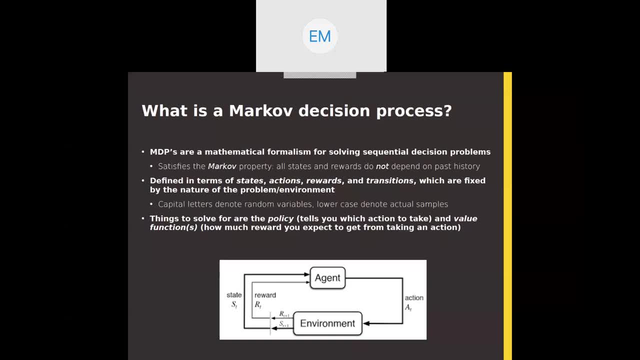 it like you could have to make multiple decisions, one after another, leading you to some unknown state, and it's called a Markov decision process because it satisfies the Markov property, which is that all the states and words do not depend on past history. so if you're, you're in a current state and 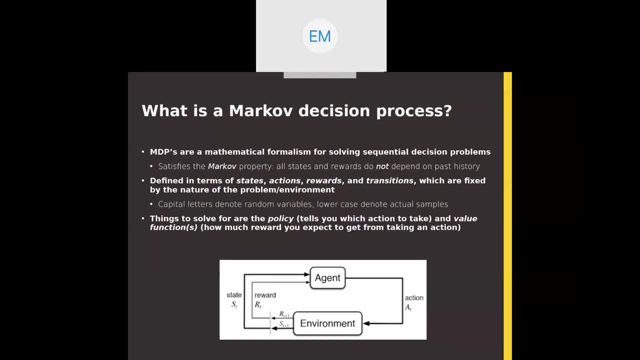 you're trying to decide what, what action you want to take. it doesn't matter how you got to that state. all that matters is like what that state is and uh and what states you can get to from that state. so it doesn't matter about the history and 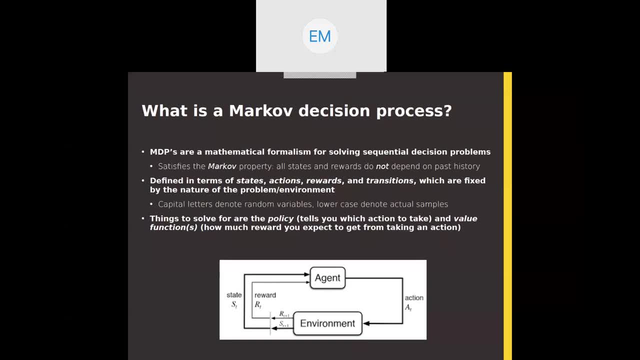 if you do have a problem that does kind of seem like it depends on your past history, usually there are like tricks that you can use to like change things around, uh, to make it so that it doesn't. um, the simplest trick is to just use the past as your current state. 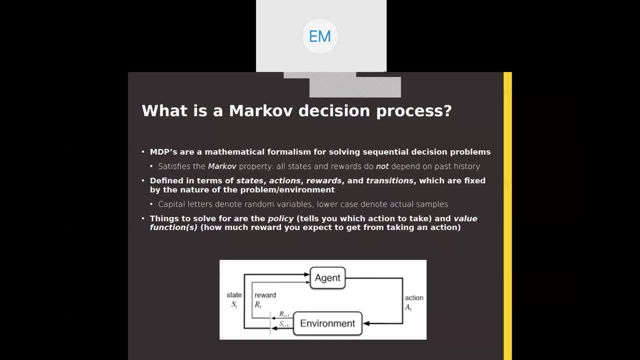 it's kind of a cheap way of doing that, but it works, and so all the inputs that you're going to have into the Markov decision process are states, actions, rewards and transitions, and once you have all of these things defined, that sort of like defines the scenario that you 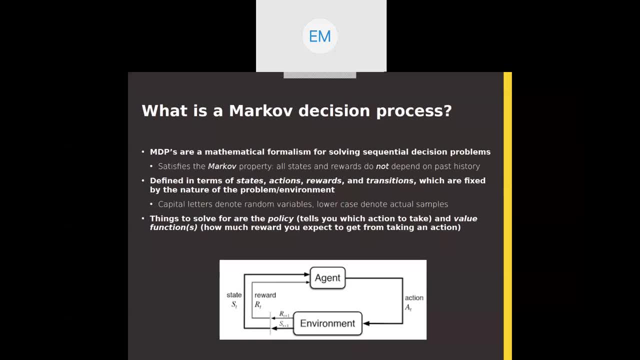 have and what you know, what rewards you, what potential rewards you could get out of this problem you set up, and once you have all those, you can then use those to solve for two other things: which is the policy, which tells you what action you need to take when you're in a certain state, and the second thing is the a value function. 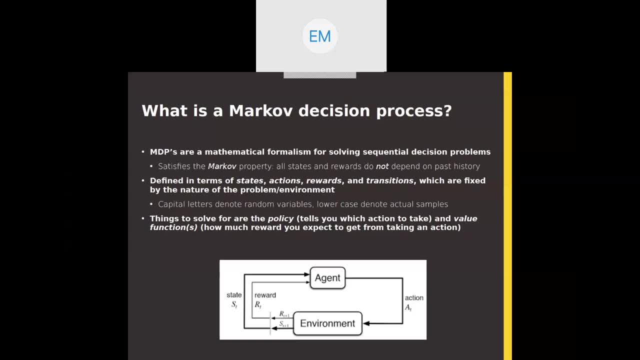 which tells you: if you do take this action, how much reward do you expect to get from taking that action? down here in the bottom you can see it's kind of like the prototypical feedback of MDP, user reinforcement learning. we start off with agent, which agent is just like the algorithm for solving. 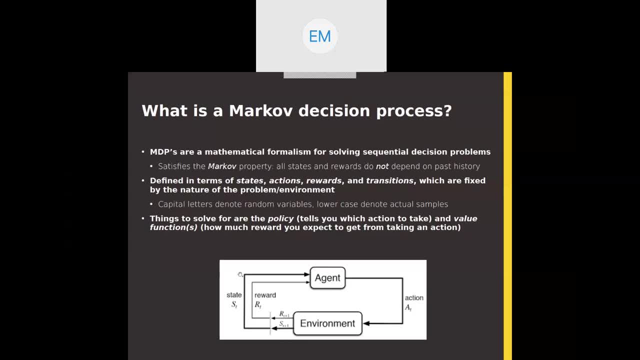 the MVP or that you can think of as the policy it takes in a state and spits out an action. it's like what do you do in your current state? that action influences the environment somehow and update causes it to update a state and one step into the future, and then the agent takes that new. 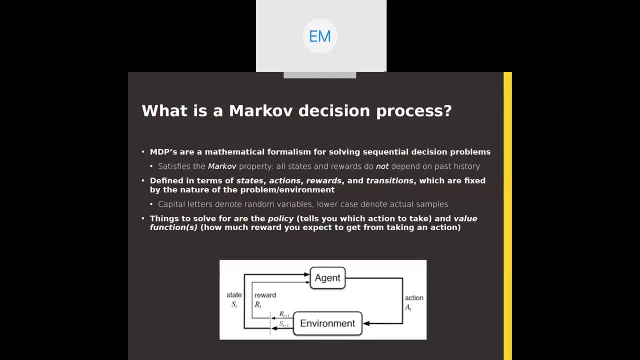 state and decides what to do from that point on. so it goes round and round, continuously updating Estates and taking actions, and there's also a reward which kind of tells you how close you're getting to your goal- and I'll have more to say on that in a second. 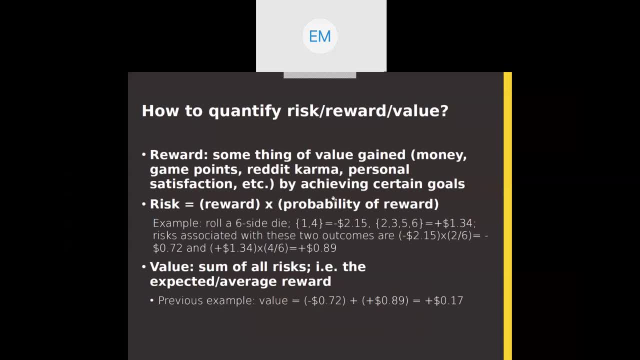 so let's start quantifying these things first and talk about the- uh, risk and reward and value, which are all kind of different pieces of the same thing. so the- the reward- is fairly obvious. uh, it's just something that you want to Maximize. it could be very general, it could be whatever. 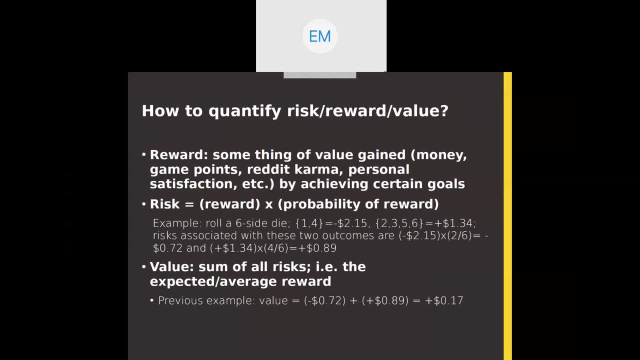 thing you're trying to get the most of. it could be money. it could be points in a game, Reddit, Karma, just like how happy you are in your life- pretty much anything. anything you can put a number on here like I want to Maximize this. the risk is uh, counter to what most people. 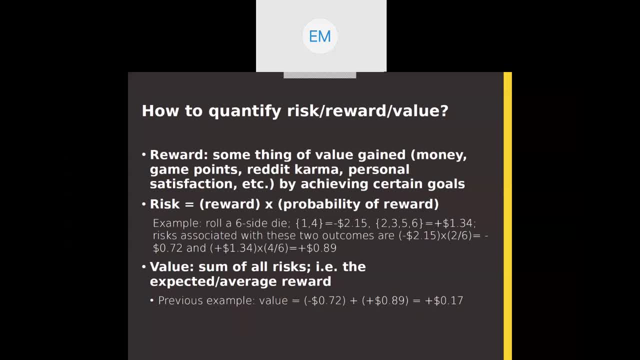 think of as risk, is near risk kind of has a negative connotation. risk in the mathematical sense is kind of like. it's kind of like the reward that you expect to get weighted by the probability that you'll actually get it. it's literally just multiply those two numbers together, so I have a. 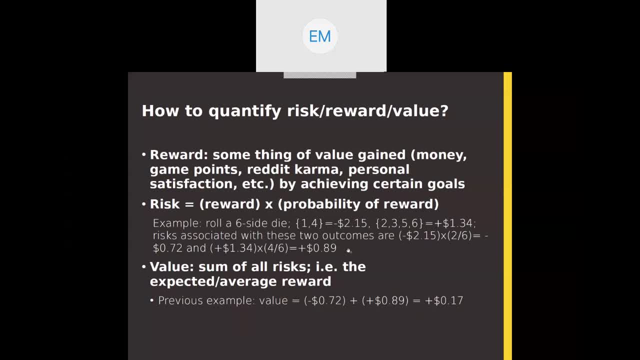 small example here, which is you roll a six-sided die on two of the sides, one on the floor, you lose. you lose some money- two dollars and fifteen cents- and then on the other four sides you gain a little bit of money, and so the risks associated with those two. you can see it's. 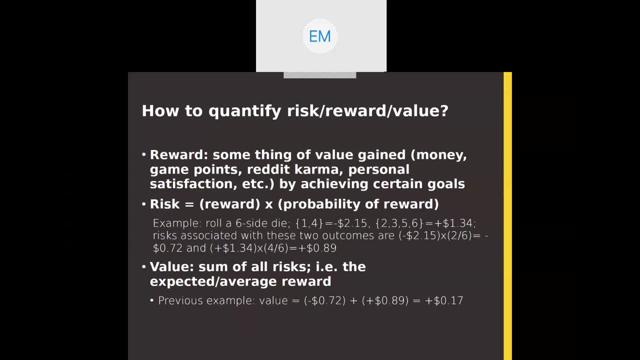 literally just. you just multiply the two numbers together, just how much reward you expect to get, and I don't think I mentioned this before. but reward can also be negative- negative rewards if something bad happens. so you multiply the reward by the probability of that reward occurring and then the value. 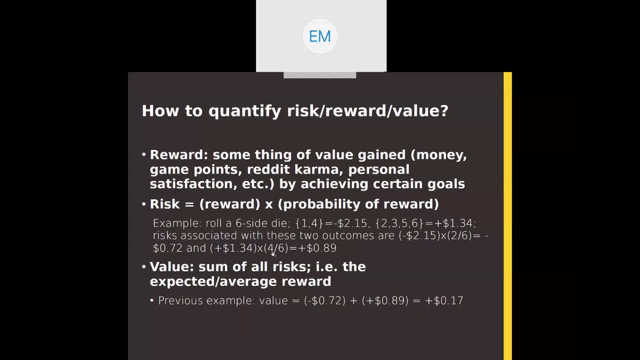 sum of all the risks involved. so the example here: you just sum two risks: 72 cents, you're negative 72 cents plus 89 cents and you get 17 cents, and so the value of 17 cents is like on average. if you play this game of rolling this dice, how much money do you expect to win 17 cents? 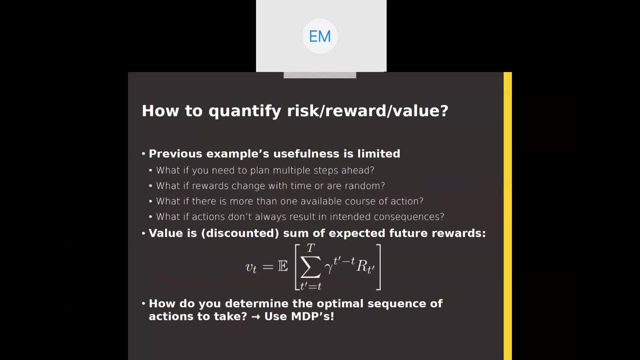 so, uh, I guess the previous slide was kind of like: simplified example is kind of limited usefulness. there are a lot of other ways that could be generalized, like but if you need to plan multiple steps ahead. the previous problem was kind of simple where it was just like: you roll a, roll a single die, but what if you're like going through a maze? you need to. 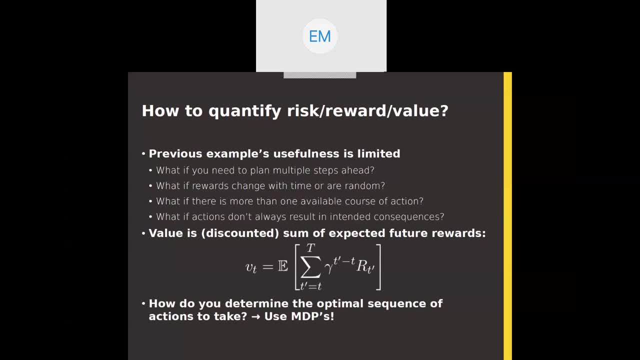 know to turn left, followed by right, followed by left, and another left, and so on. um, what if the rewards change with time or random? trying to think of a realist, maybe you're playing a game where, like, flip a coin, like even if you get heads, maybe 50 of the time you get a dollar and 50 of the time you only get 50 cents you could have. 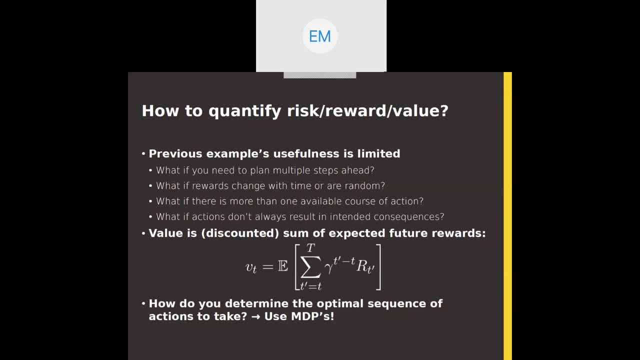 random rewards that aren't aren't fixed. there could be multiple courses of actions instead of just choosing between flip the coin or don't flip the coin. it could be like: do I go left, right forward? you could even have like continuous action spaces, like: so you're driving a car, for example, turning the steering wheel would. 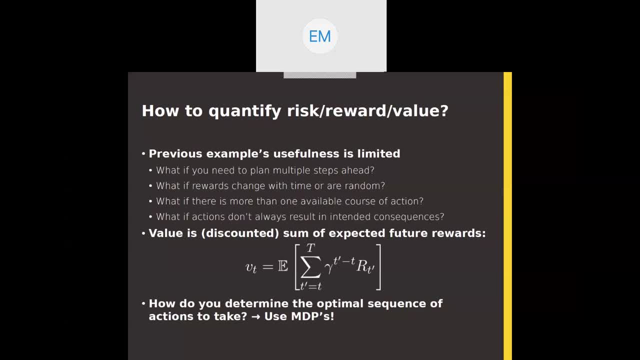 be like: turn it 10 degrees or 15 degrees or 20 degrees, any, any angle. and then final one, which is the most weird to think about. it's like: what if, uh, what if your actions don't always result the intended consequences? what if, uh, what if, by taking a certain action, you could end up in any one of 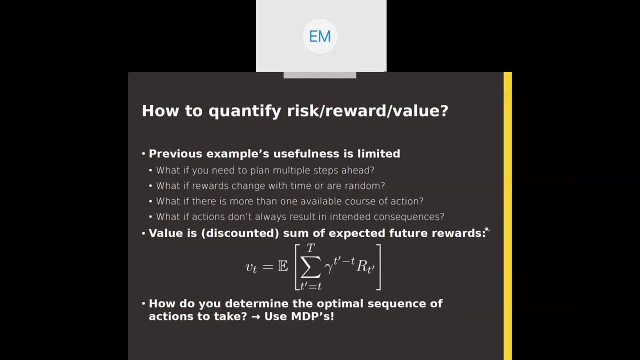 multiple states, you don't really know what the result of your actions. so we can use mdps to kind of take care of all this stuff like it's just naturally taken care of in the within the framework. and to do that we need to like generalize our idea of value so that rather than just the being 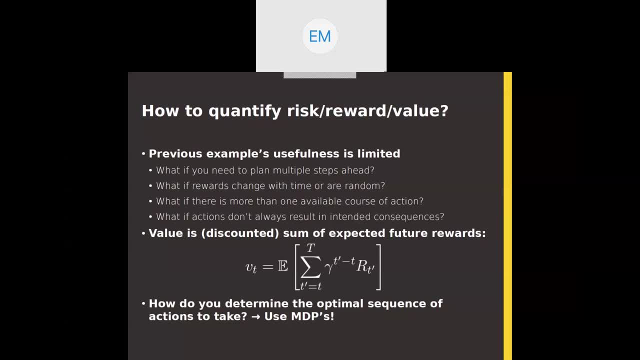 the reward that we get from taking an action. it's going to be the sum of all future rewards that we get from now up until some point in the future, which could be like maybe we stopped playing the game, or it could even be like Infinity. it's far, far far into the future. uh, you can see from this. 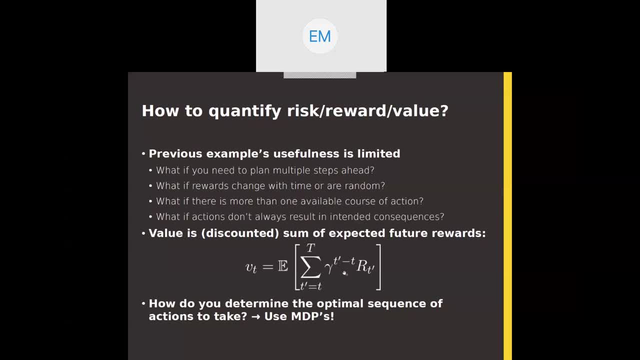 equation if you just ignore this Gamma thing right now. but if you ignore a Gamma, then you can see the value is the expectation of the sum of all the rewards, and I'll talk about the Gamma later, but it's, it's kind of like a mathematical trick to make things converge, all right. so if you have all that, how do you figure out the optimal? 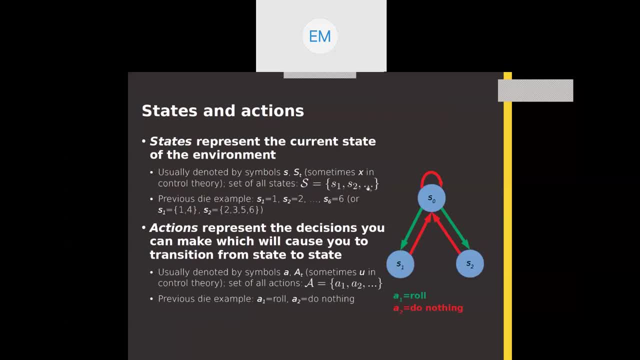 sequence: faction stick use: mdps. so, getting into some of the nuts and bolts of the inputs, I have two slides on like the inputs that you need and then other two slides on like the outputs. uh, so the first two pieces that you need are states and actions, and so I'm going to take that rolling the die example from a couple slides previous and 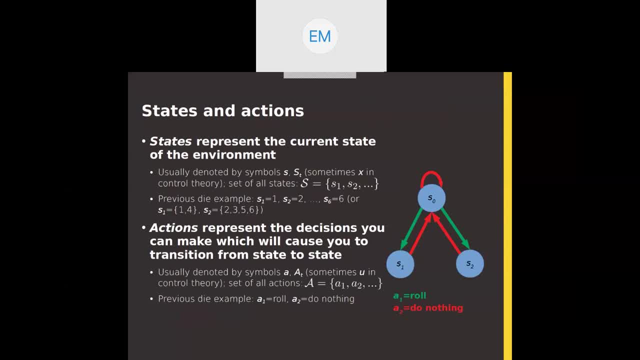 kind of just flesh that out a bit more. so let's say you have, you have that dice rolling example as your, as your mdp, your states- there's a little bit of flexibility here because you could, you could say all of your states are like just for individual sides of the die, so like you could have a state for if you roll one, you could. 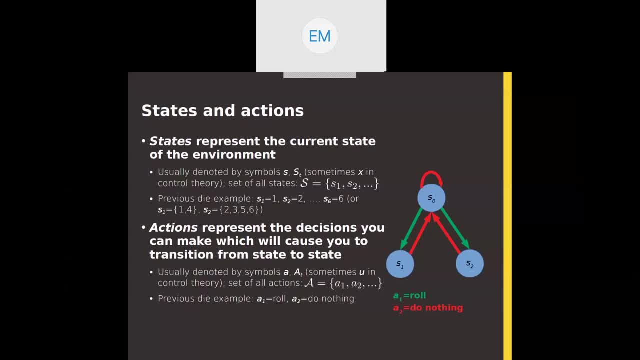 have. you could end up in the state where you roll a two, you could end up in the state where you roll a three, so on and so forth. but you can also choose to kind of like compactify that representation and make it like a little easier to work with. so in this case, since two of the sides always have 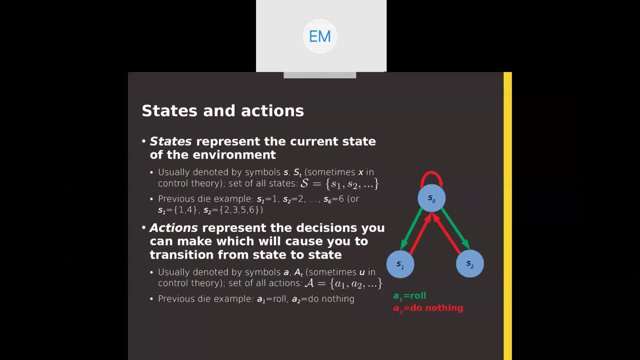 the payout and the other four sides always have the same layout and I just like threw them all together in the same same state because there's really no difference between them. so you can see. I called the the state where you roll either one or four s1 and the state where you roll any of the. 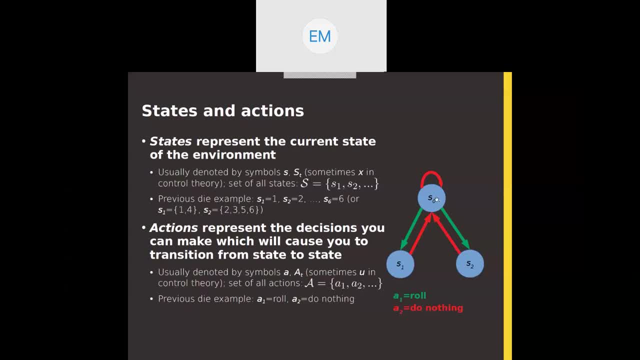 other four numbers, s2, and I have kind of a graphical example over here on the right. so three, three different states. zero is actually the state where, like you haven't rolled anything here, it's like the starting state, and the way that you transition between these states is obviously by taking actions. 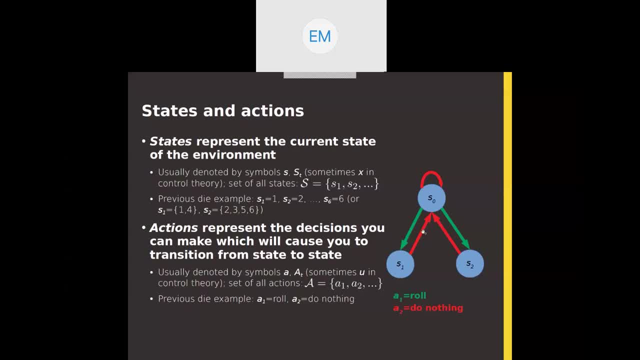 so the actions in this case are edges between the states and in this, this dice rolling game that we're playing, there's only two accents. there's either do nothing or roll right. and so that defined the two, two actions that you have, and by choosing one or the other you can transition between the 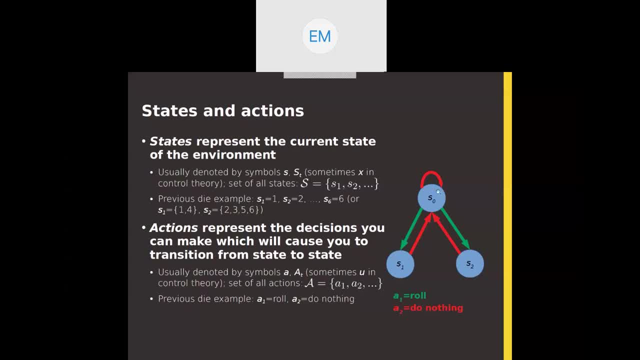 states there are only certain transitions allowed. so, for example, let's say you start in state s0. if you do do nothing, you just end up. you know you're just sitting there doing nothing, so you just end up back in the same state and start at the. success is the top loop if you decide to uh, roll, roll the. 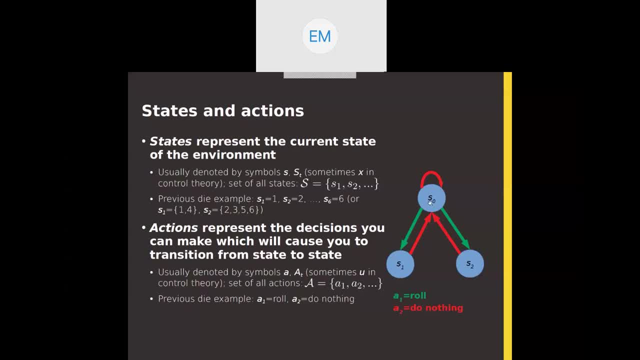 die. um, now, this is a case where, uh, your action could have unintended consequences, right, because, uh, you roll the die, but there's two potential states that you could end up in by making this choice. so you can either transition from s0 to s1, or you can transition from s0 to s2 along those green edges and then, once you're in, 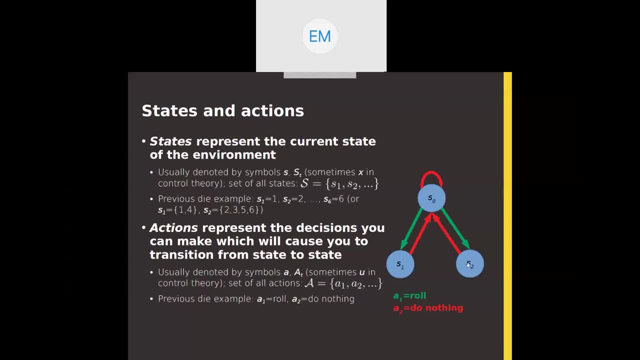 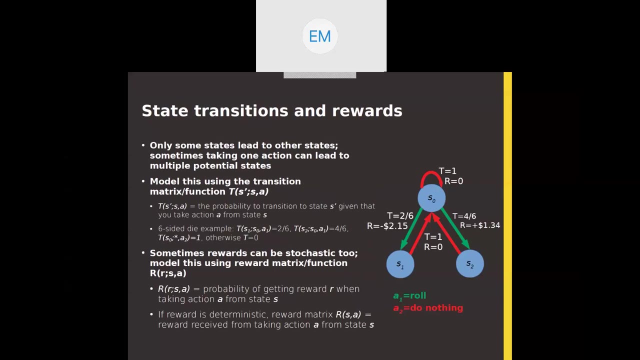 either one of those two states, you can just do nothing, and then the product, the scenario, resets and then you go back up to the status here. so those are the first two pieces. the next two pieces kind of uh, kind of build on top of actions and states and like the transitions that between them. so the first thing is like it's technically 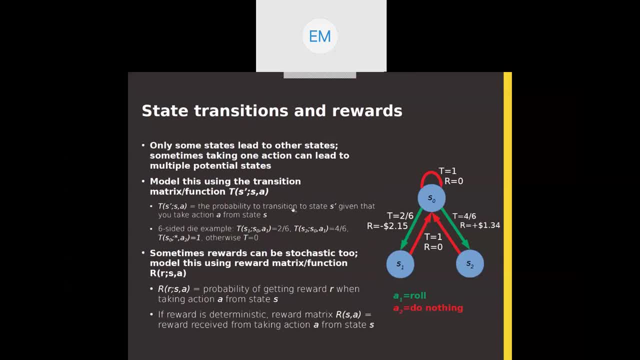 third thing is the transition function, or transition Matrix, in case you have discrete states. so, uh, I wish I could highlight this, but, uh, as you can see over here, it's a tssa. so this is the transition function and you can think of it as the probability to transition from state s, your original state, to 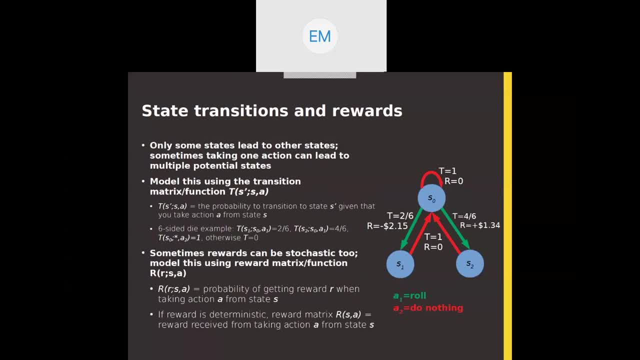 a new state s prime by taking action, a. so you plug all three of those things in old state, new state and the action that you take, and this will spit out what's the probability of that happening. um, and you can see in the, so I've kind of spelled it out for the, the example that we have. you can. 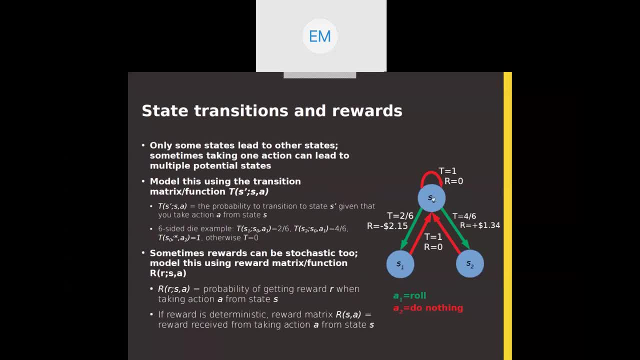 see that if you start in s0 and you take action a1, which is to roll the dice, and the probability of you ending up in state s1 is two, six, because there's only two out of the six sides- uh, you, there's also a probability of the end. 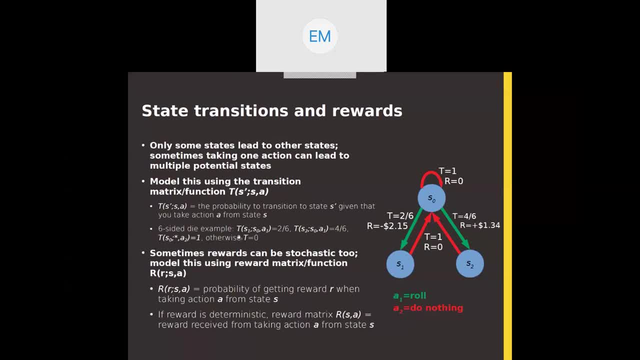 probability four, six and then the reverse, going back up to state s0. you can get to s0 from any one of the states by taking the do nothing action. that's what that star means: wild card. you can do anything or you can start from anywhere, and then all the other transitions are zero. so like 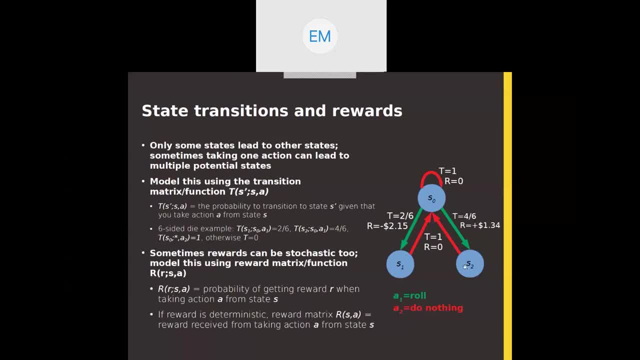 there's, there's no probability. there's no way that you can get from s1 to s2, right, uh, there's no way that you can get from s0 to s1 if you do nothing, so those transition Matrix elements will be zero. um, next thing, uh, the final thing that you need will be your reward. 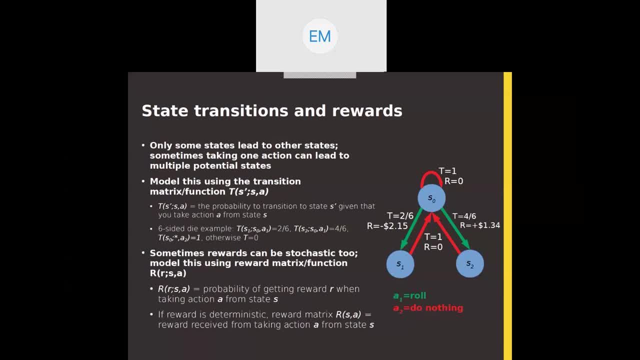 function. so this tells you how much reward you will get out of like doing the action or getting to the state or whatever. there's two different forms for it. there's- uh, this is stochastic form- and deterministic form. so the stochastic form is pretty similar to the transition function. it's 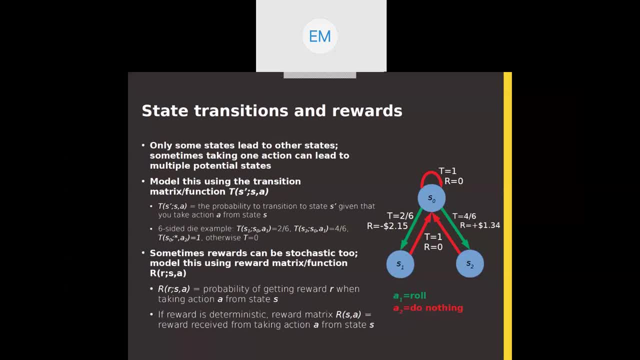 a probability distribution over the rewards that you would get if you start off in state s and take action A. so start in S, take action A. maybe there's like 10 different rewards you could possibly get, and this one assigns a probability to each one of those 10 if your reward is deterministic. so 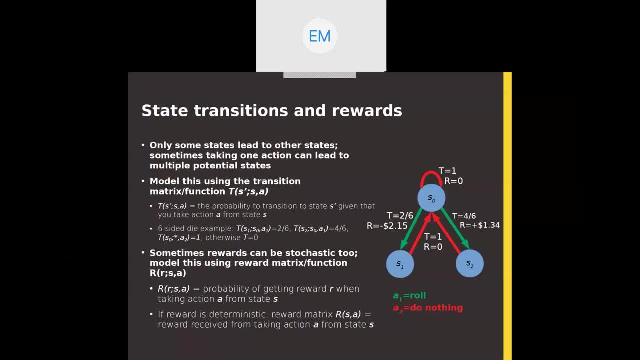 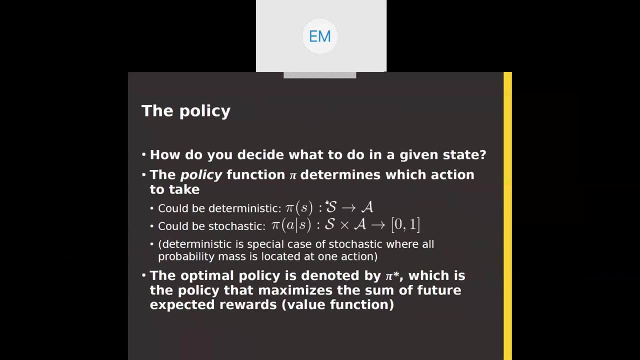 like you know, if I'm going to take take this, take this action in this state, I'll get this reward. then you don't need to involve probability in it and this will just be like a regular function that'll spit out the reward that you get. okay, and then now, now that you've defined all four of those things- states, actions, transitions. 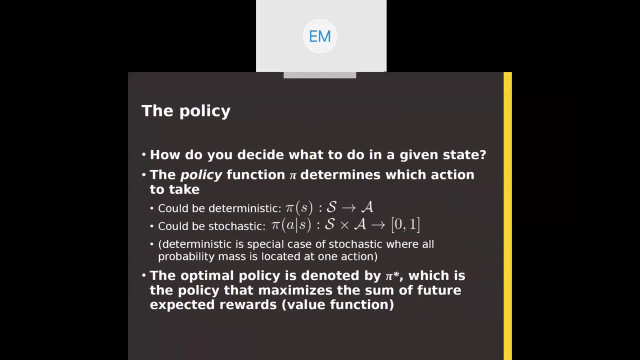 and rewards. now you can actually. that defines the whole mdp, and now you can solve it. so, um, just to recap the, the two things that you get out as part of the solution are policy, which tells you what actions you need to take, and then the value function, which tells you how valuable your actions. 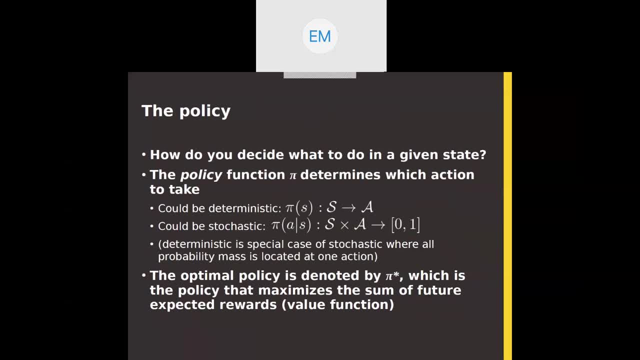 are or how valuable your states are. so policy here, which is usually denoted by a pie. there's also two different cases for this, one which kind of parallels the um, a reward function. it could be either deterministic or stochastic. in the deterministic case you just have a simple: Okay, I'm in this state, what do I do? and so just maps a state to an action. 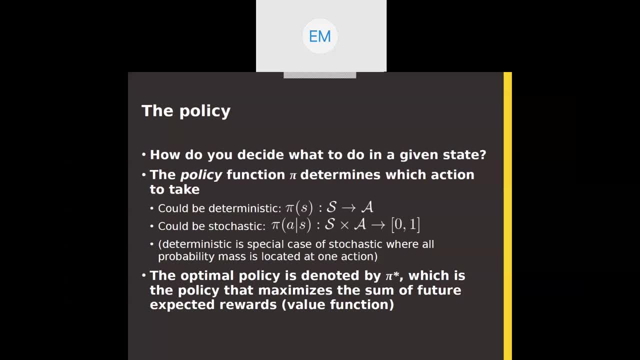 or you could also be stochastic, which is like, okay, I'm in this state. you know, maybe my knowledge of what's going to happen in the future isn't a hundred percent perfect, so maybe there's a 10% probability that I go this way and a 30% probability that I go this way. 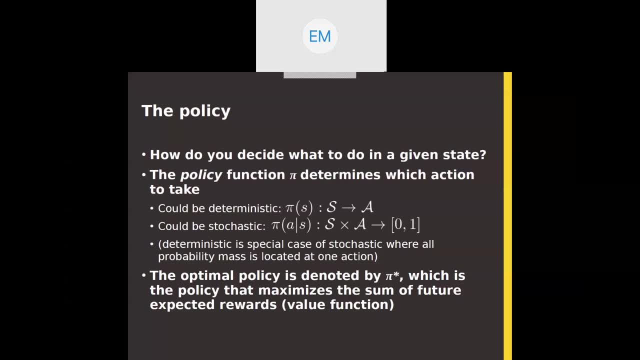 and a 60% probability that I go some other way. When you make your decision you just kind of sample that probability distribution So you can go either way. And just to note there are many different policies for any given problem. like the MDP that describes my life. 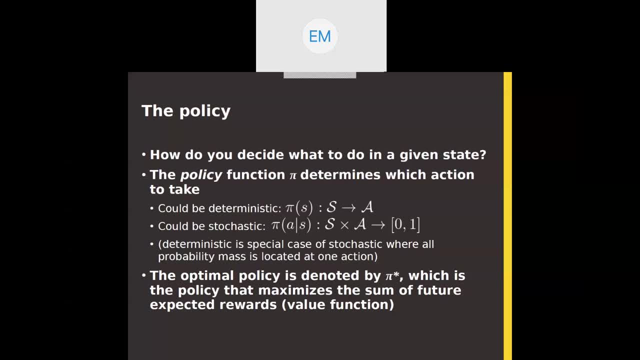 My policy could have said: don't go to work today, just stay in bed, But the optimal policy probably involves going to work. So there's many different policies, but only I wanted to say there was only one, but there could actually be multiple optimal policies. 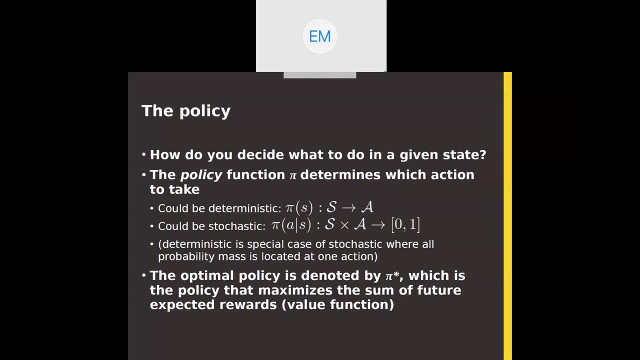 They're all. maybe they're slightly different, slightly different decisions that lead to the same result, but they're the same. There is some truly optimal policy which will optimize and maximize the reward that you're looking for. That optimal policy, or the set of optimal policies. 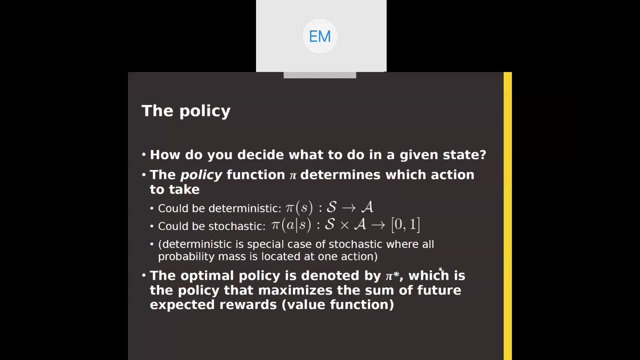 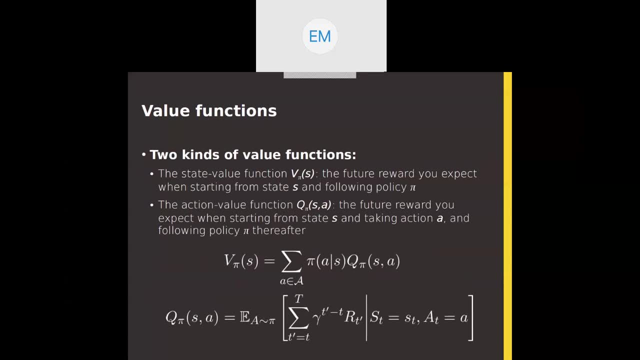 is usually denoted by this pi star. And then, finally, the second piece that you get out of the MDP solution is the value function, And so this tells you, like what sort of reward that you can expect to get From either being in a state or getting to the state. 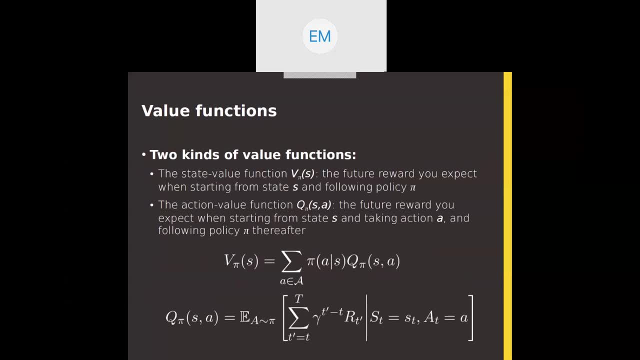 or even if you're like in a state and you have multiple actions, what's, how much reward do you expect from taking action one versus action two versus action three? So there's two different flavors of this. There's the state value function BS. 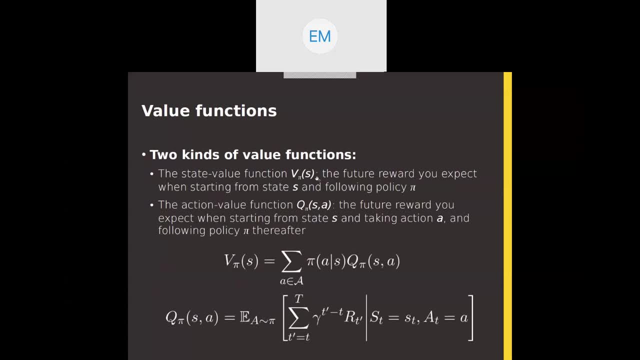 and also important to note that this is a function of the policy. So if you're using like a not optimal policy, then you'll get a sub-optimal value function right. Maybe your policy is just terrible, So your value function will be very low. 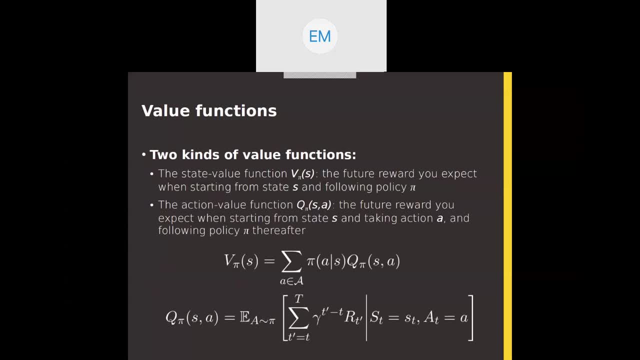 but if you have an optimal policy that you're using, then your value function can be very high because you're getting a lot of reward. So yeah, there's the two flavors. There's the one that just directly maps states to values. That's just like I'm in this state. 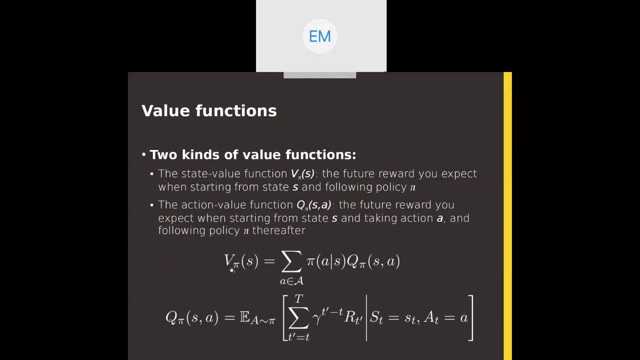 If I follow this policy, all right, how much reward do I expect to get? And then the other flavor is this Q, which is the action value function or state action value function. Most people just call it the Q function, But so that maps from states and actions. 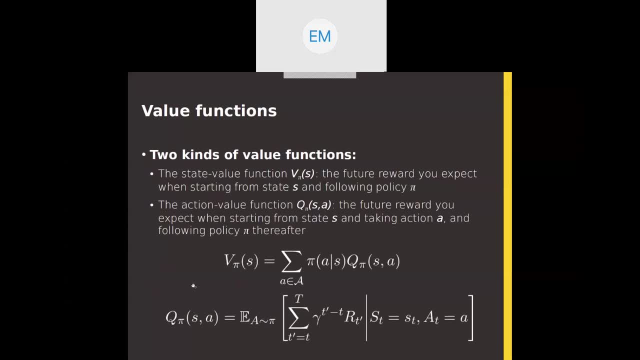 to rewards given the policy. So that's like, if you're in this state, how much reward do I expect from going left, going right, going forward? You just plug in different, different actions and then that'll give you the reward for this, the expected future reward. 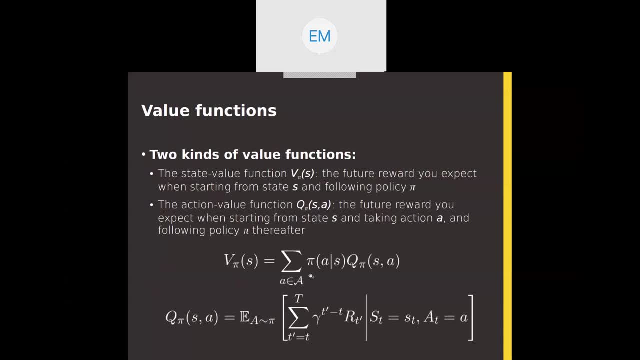 for those different choices. And you can see in the bottom is a kind of a callback to the original value function that I defined, like five slides ago, which is that sum over discounted rewards. So you can see this, you can see this callback to like the value. 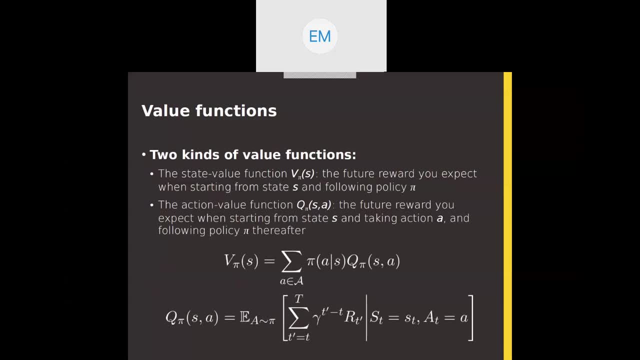 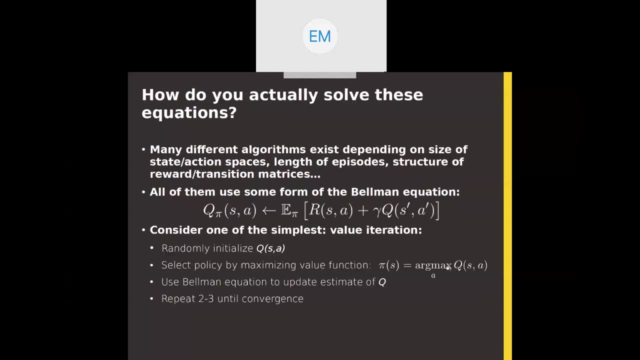 that you get out of the state is going to be the sum of all the rewards that you, that you would potentially get in the future. Okay, So that that sets up all the everything like, all this stuff you need to know to solve the problem. 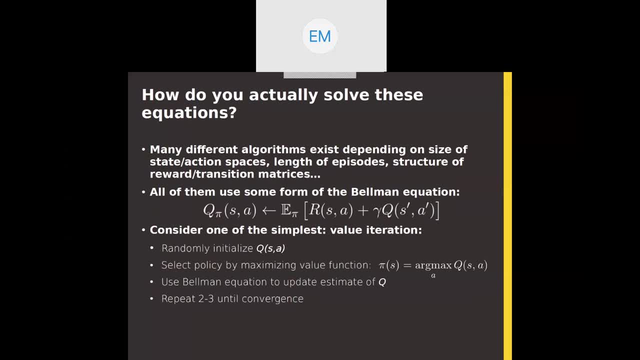 but how do you actually solve it? Okay, All right, So there's actually like a million different ways to solve it And it depends on, like, how complicated your problem is, whether the state space is continuous or discrete and whether your action space is continuous or discrete. 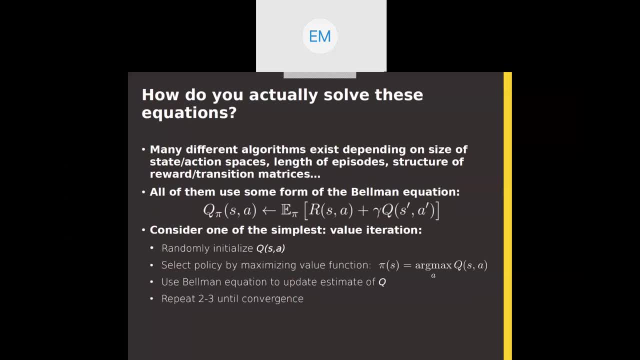 all sorts of different, different things, But one thing that they all have in common is that they use some form of this, this update equation here, which is called the Bellman equation or the Bellman Optimality equation, And so this describes. 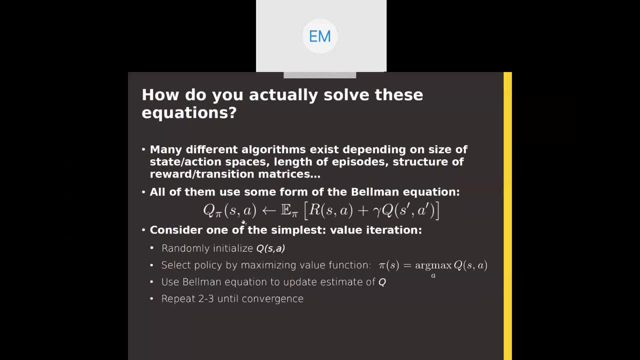 this describes how you like update your estimate for the value of being in a state given. As you like explore through an environment. This is really relevant to the reinforcement whipped too. just just like a high level On the right hand side you can see like our. 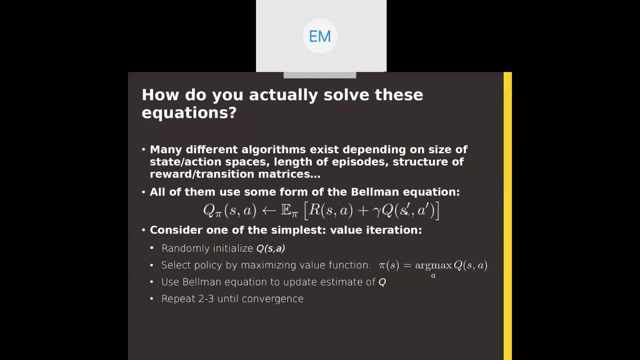 which is more focused on, and that Q and Q1, which is our value function. and so, and then on the left, you can see the Q function again. so this is what this is saying: is like the value function, the value of being in state s and taking action. a is equal to like the expected. 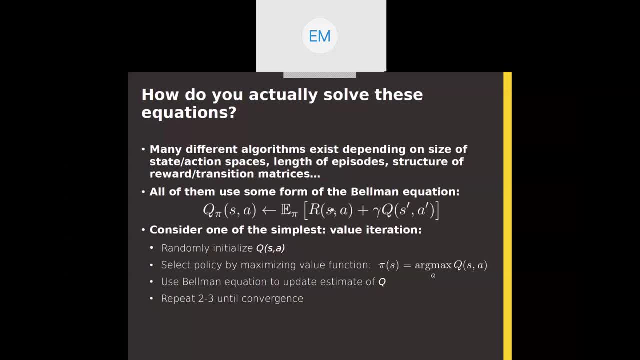 value of the reward that you would get on that next time step, plus all of the rewards going forward from. from that point, you can think of it like so, here's. so you're gonna take like ten time steps, the Q on the right with the s prime, and 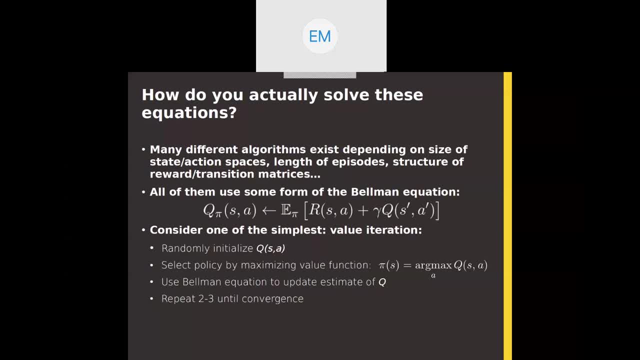 the a prime. that represents the value that you get taking like the final nine time steps. R represents the value that you get from taking very first time step and then you just add them together and then that gives you how much, how much value you expect to get from. 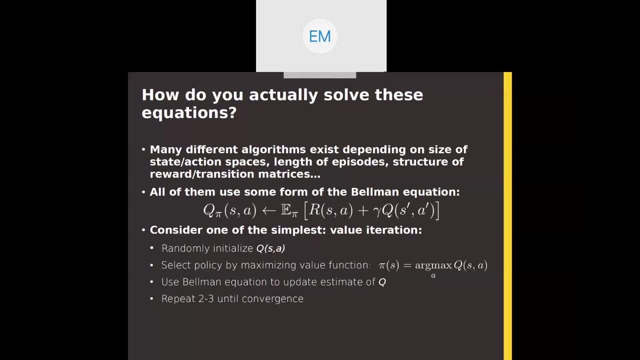 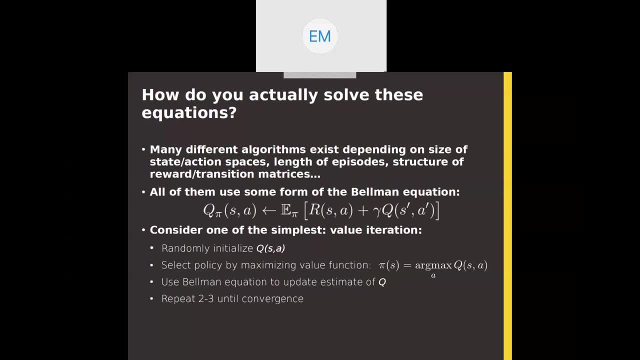 the beginning, right? so it adds that one time plus the final nine times steps. so time plus the final nine times steps. so time plus the final nine times steps. so they all, all of the algorithms utilize. they all, all of the algorithms utilize. they all, all of the algorithms utilize this updated version in some form or 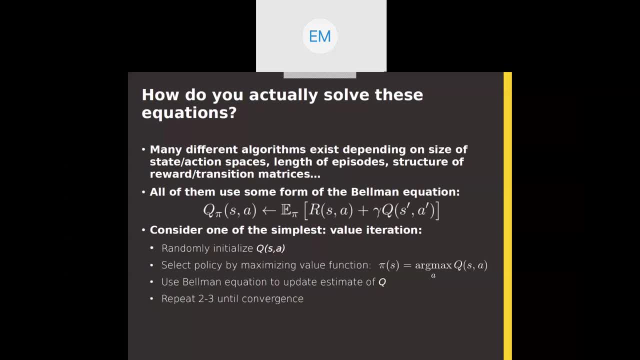 this updated version in some form, or this updated version in some form, or another, another, another, um. you know various levels of um. you know various levels of um. you know various levels of complication: um, we're gonna go pick I'm. complication, um, we're gonna go pick I'm. 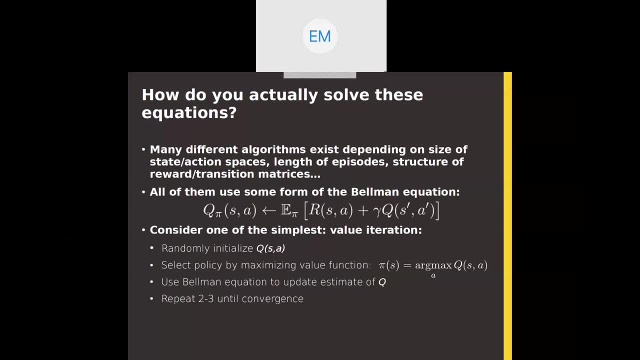 complication. um, we're gonna go pick- I'm gonna pick one of the simplest ones here, gonna pick one of the simplest ones here, gonna pick one of the simplest ones here, which is called value iteration, which is called value iteration, which is called value iteration, and it's, it's simplest, the simplest one. 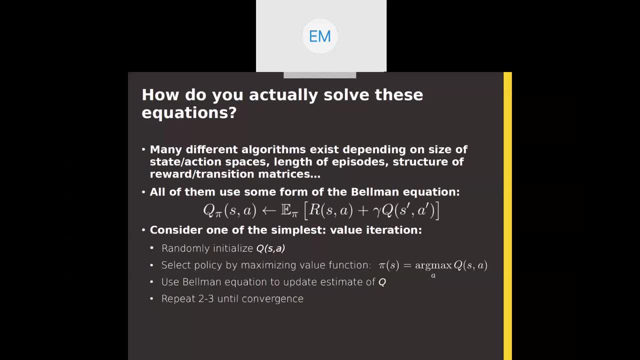 and it's it's simplest, the simplest one, and it's it's simplest, the simplest one to like think about. but it's actually to like think about, but it's actually to like think about, but it's actually like a really terrible one from a, like a really terrible one from a. 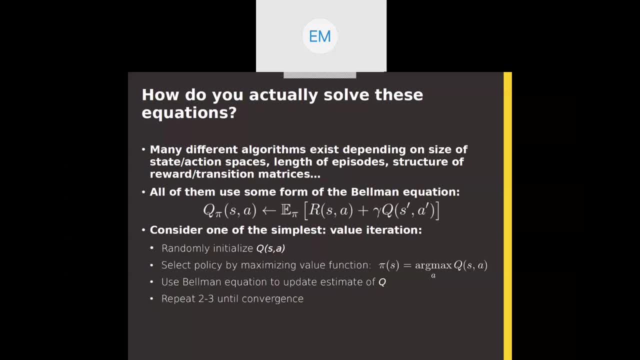 like a really terrible one from a computational efficiency standpoint. so computational efficiency standpoint, so computational efficiency standpoint. so you might not want to use it in. you might not want to use it in, you might not want to use it in practice, practice, practice. but the way it works is you initially. 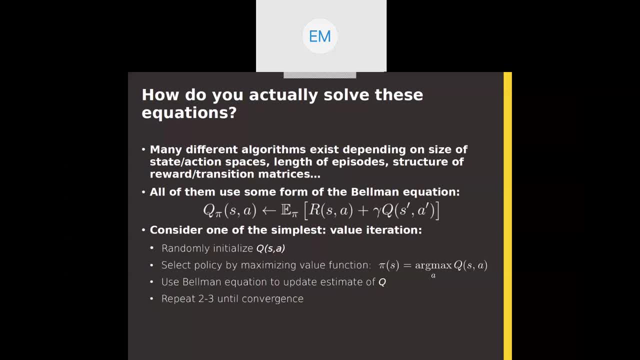 but the way it works is you initially. but the way it works is you initially. you start out with some random. you start out with some random, you start out with some random queue. so this is like your estimate for queue. so this is like your estimate for queue. so this is like your estimate for by maximizing the value function. so 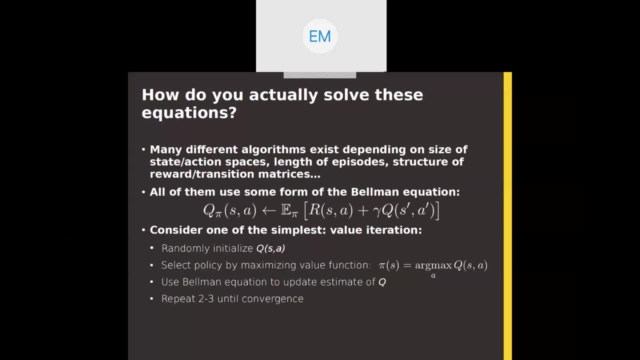 by maximizing the value function. so, by maximizing the value function. so, based on your current understanding, based on your current understanding, based on your current understanding, what's the best possible course of? what's the best possible course of? what's the best possible course of action, action, action. so you figure that out. 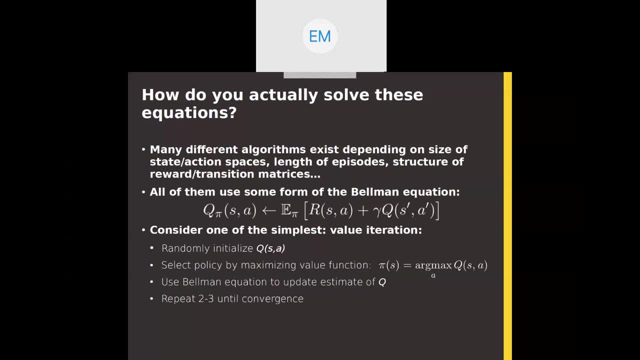 so you figure that out, so you figure that out, and then you use the bellman equation, and then you use the bellman equation, and then you use the bellman equation to update your estimate of q, so even to update your estimate of q, so even to update your estimate of q, so even though your initial estimate was, 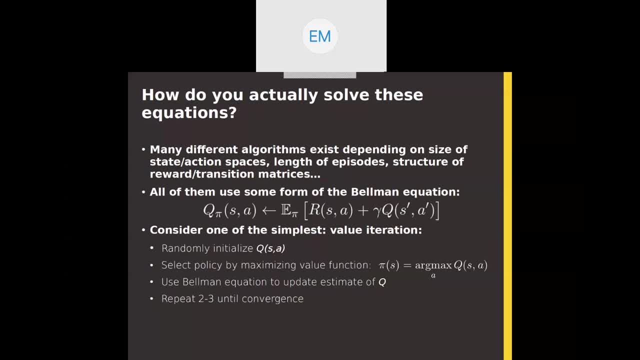 though your initial estimate was, though your initial estimate was terrible, terrible, terrible. by using the bellman equation you can, by using the bellman equation, you can, by using the bellman equation, you can kind of make it like a little bit better, kind of make it like a little bit better. 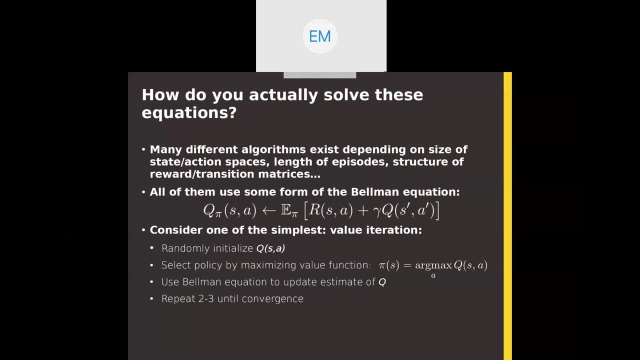 kind of make it like a little bit better, and then you just do that over and over, and then you just do that over and over, and then you just do that over and over again until convergence, until the q again, until convergence, until the q, again, until convergence, until the q value stops changing. so, even though 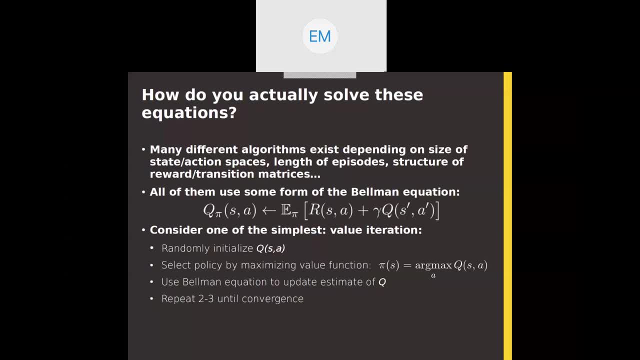 value stops changing. so, even though value stops changing. so, even though, even though you started, it was just like. even though you started, it was just like. even though you started, it was just like: worst possible, totally random behavior. worst possible totally random behavior, worst possible totally random behavior, simply. 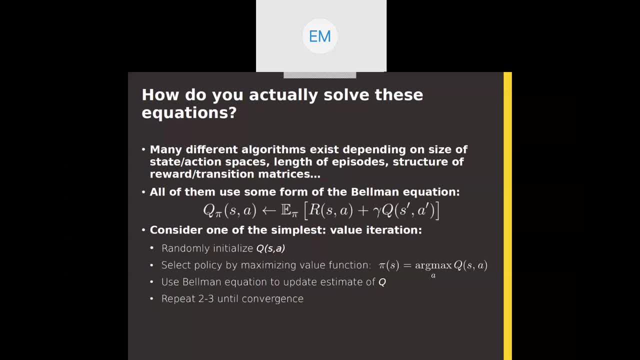 simply, simply, by iteratively using the spellman, by iteratively using the spellman, by iteratively using the spellman, equation, you just slowly, slowly made it equation. you just slowly, slowly made it equation. you just slowly, slowly, made it better and better and better until better and better and better until. 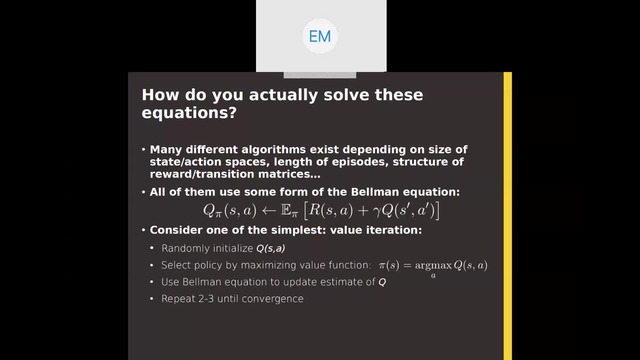 better and better and better until eventually you've reached the optimal. eventually you've reached the optimal, eventually you've reached the optimal optimal policy, and it optimal policy, and it optimal policy, and it. it's been proven that this, this will. it's been proven that this, this will. 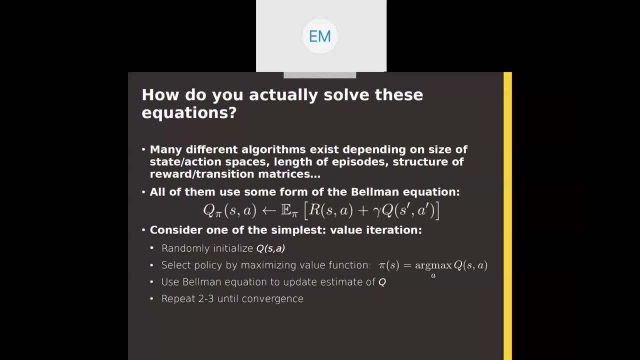 it's been proven that this, this will always work, always work, always work, given infinite time, of course, given infinite time, of course, given infinite time, of course, in some cases, in some cases, in some cases. so, if you have a small enough problem, so, if you have a small enough problem, 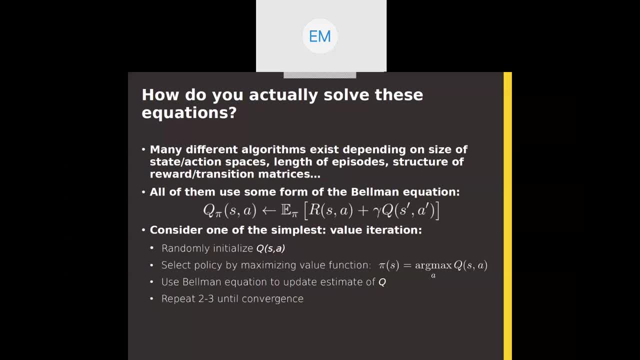 so if you have a small enough problem, then then then infinite you can cut it off at like a infinite you can cut it off at like a infinite. you can cut it off at like a finite number of time steps. finite number of time steps. it'll be fine, it'll be close enough, but for like really complicated problems, this will never work. 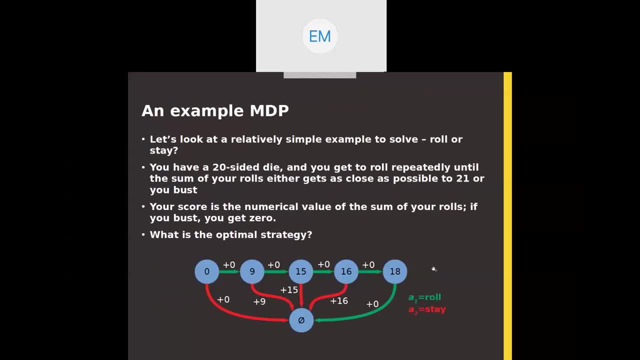 but for the case that we're going to go through it, it will work. uh, before i move on, are there any questions? okay, cool, i think i saw someone typing questions in the chat. i haven't been looking at it, but it'll. i'll take a look at it after the talk, okay, so? so now i have a slightly more complicated 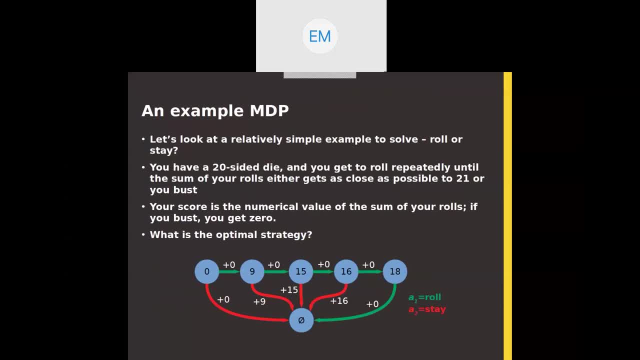 example. that'll kind of like get into the details. uh, that we that we discussed previously in more detail. um, so the way this works is it's kind of similar to the original problem. well, it's only similar in the sense that you're rolling ties, dice, but, uh, you have a d20 or a 20. 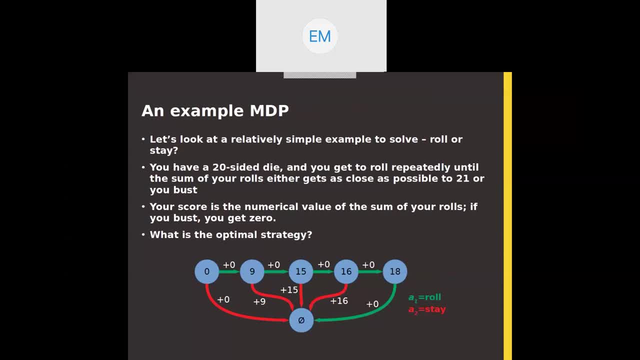 sided die and you you're basically playing blackjack with it. you just roll it over and over again and, if you get, you sum up the rolls as you go along. so like in the example, i guess, in the example image that i have down here, you start off at zero and then you roll a nine. so now your 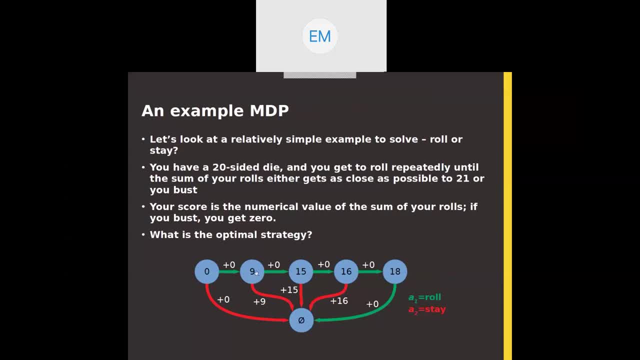 score is nine, and then you roll again, uh, you get a six. in this case you end up with 15 total. and then you roll again, you get a one, and you roll again, get an 18, and then maybe let's say: you roll again and you got like a five, so you go over 21 and you go bust. um, so yeah, so your score. 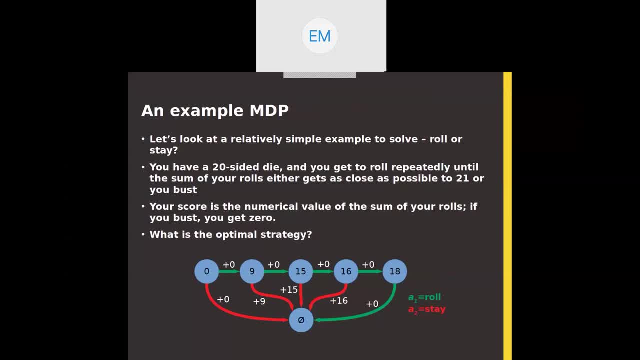 or your reward is like the numerical value of the sum of your rolls, but you can quit at any time. so, like, if i wanted to uh, once i like got to 15, i could have said, okay, that's it, i'm going to call it. you know, i don't want to, i don't want to risk going bust, so i'll just stop the game right there. 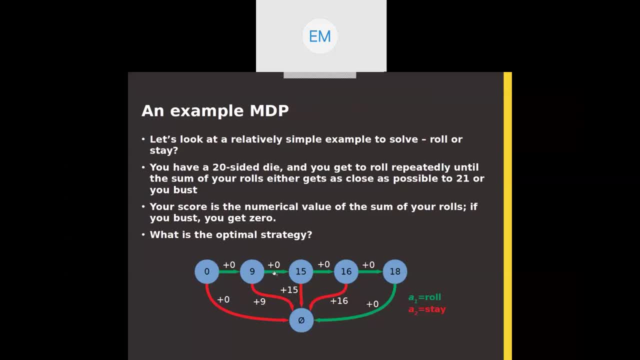 and once you stop the game or go bust you, you transition to this terminal state, which is like this all absorbing state. all states lead to it eventually, and that just means like the game is over. um, so in the- in the image you can see, i have two actions. there's the, the roll the dice action. 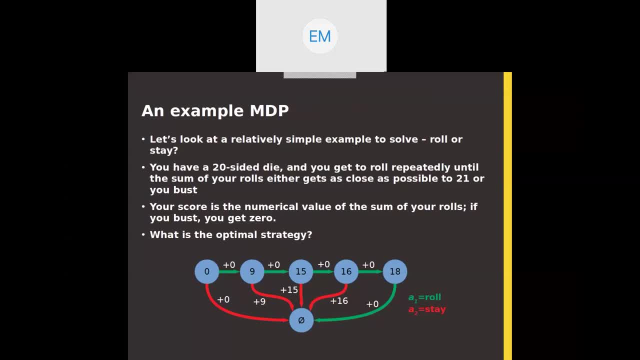 or the do nothing, stay action. i guess in this case, where you like take what you've earned so far and just leave um and the, the white numbers are the rewards that you get from the transitions, so you can see if you move left to right along like this top using the green arrows, you don't actually 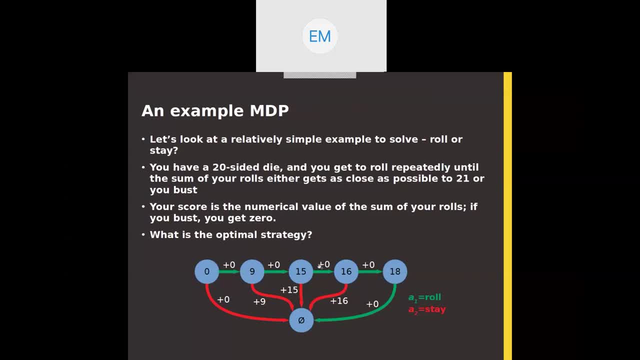 get any reward from uh, from moving along. uh, because you you haven't like finished the game yet, but once you either go bust, which you can see from like the very far right side, once you go bust you go back down the terminal state but you get zero reward. so you haven't gained any reward at 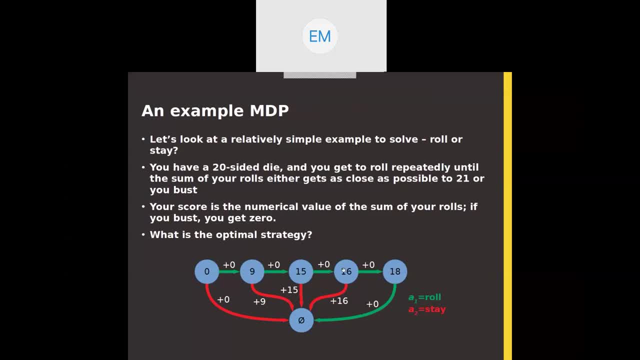 all along that trajectory. but if you say you're in like state 16 and you decide to stay there, then the game ends. but you gain 16 points, and so your total- um, yeah, your total for the game is 16.. okay, does that make sense? 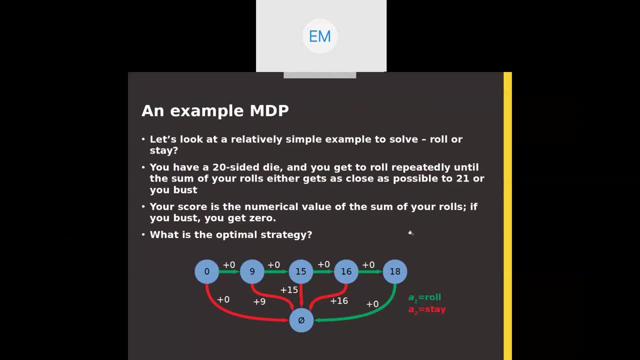 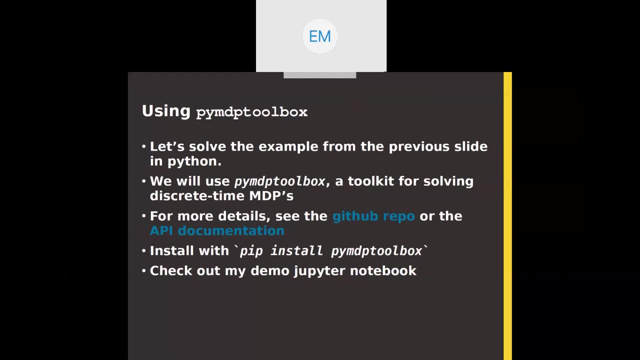 okay, so, uh, so this we're going to use as like the example to figure this out. so what is the optimal strategy? all right, so now this is. i'm going to switch over to my jupiter notebook. oh, don't look at that. that's the answer. 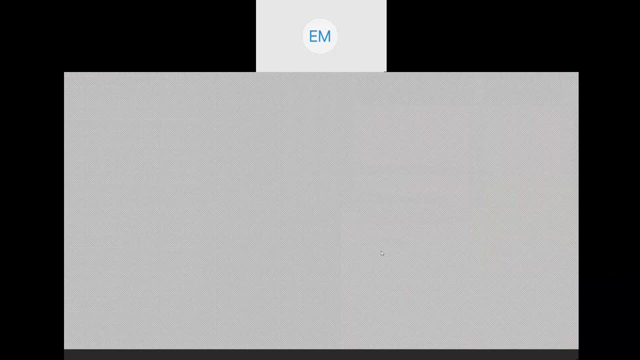 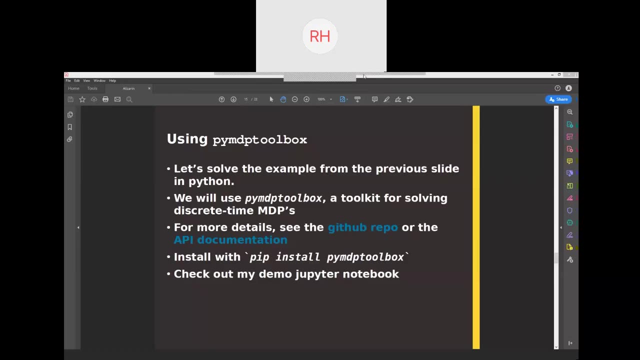 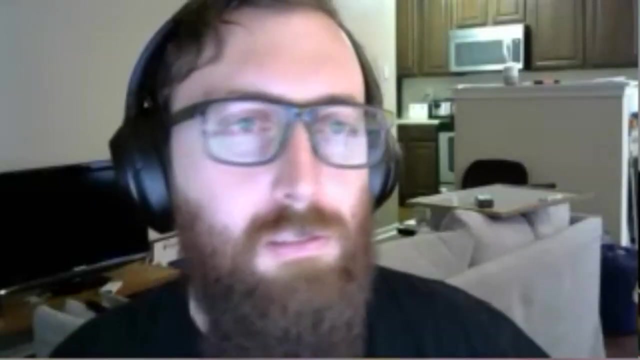 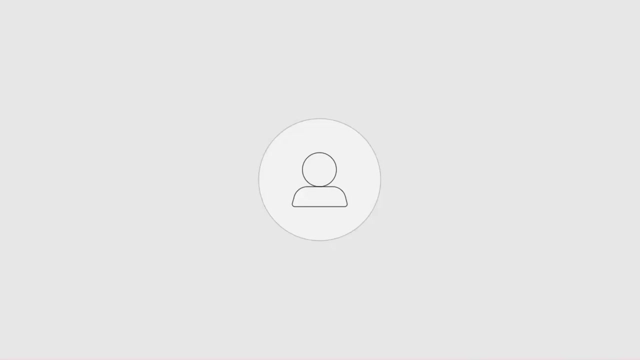 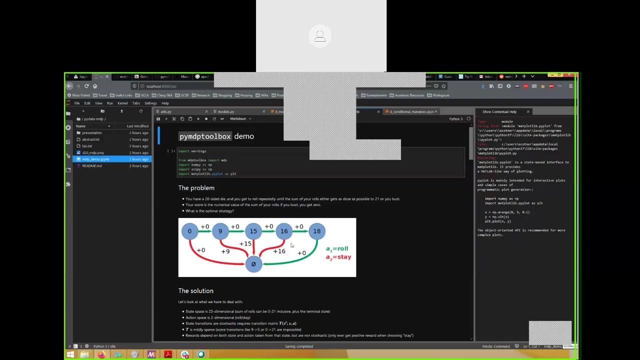 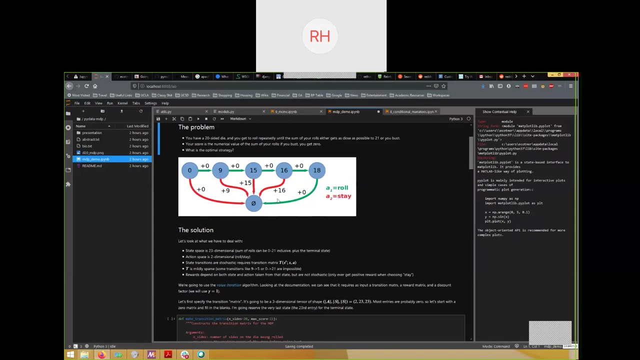 there we go. okay, that's great. i think you're just. oh, i might just be sharing the application. stop sharing and switch functions and the reward matrix, And then also a little bit of plotting. Got to visualize the solution, All right, so this just restates the problem. 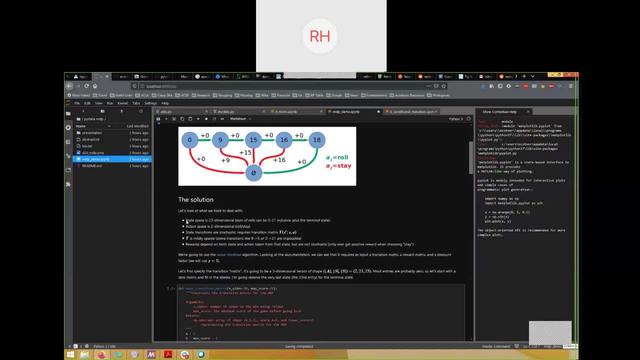 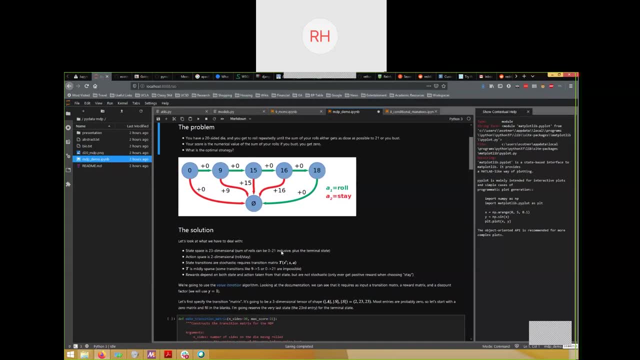 You just roll until you get bust. Little more details about the states, actions, transitions and all that. So the state space is 23-dimensional. in this case You can be in any state from 0 to 21 inclusive. So that's 22 states plus the final terminal states. 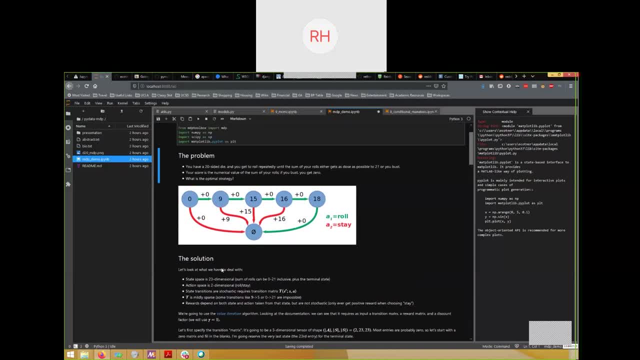 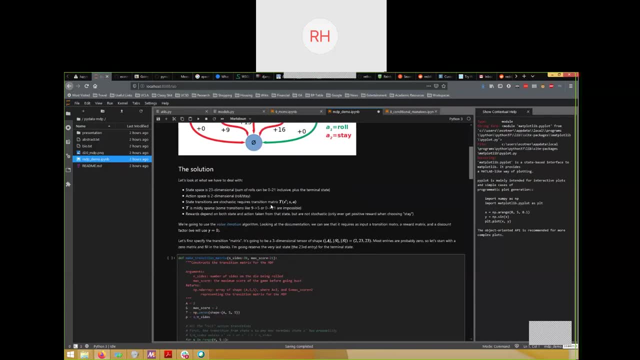 All together, that's 23.. And the action space is two-dimensional. It's just: do you roll the dice or do you not? And then the transition function, or in this case, it truly is a transition matrix, because we have a discrete number of states. 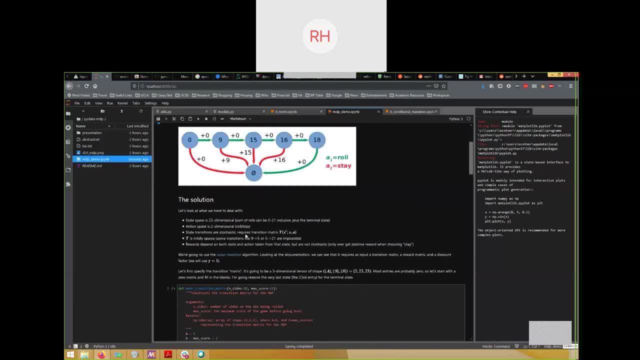 Yeah, we have that. It's mildly, It's sparse, very similar to the original example that we had, where a lot of the transitions are literally impossible. There's a way you can go backwards from 9 to 5. Or you can't go directly from 0 to 21. 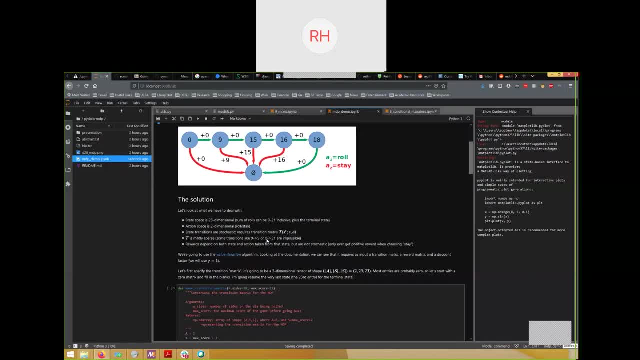 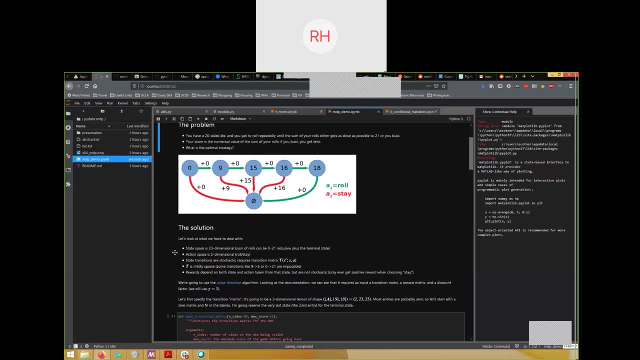 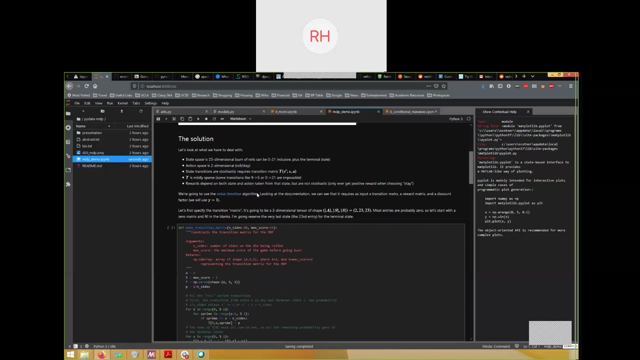 because there's no way to roll 21 on a 20-sided dice, So stuff like that is impossible And those elements in the transition matrix will be 0. And then you're going to use the value iteration algorithm, which I don't actually code up, the value iteration algorithm. 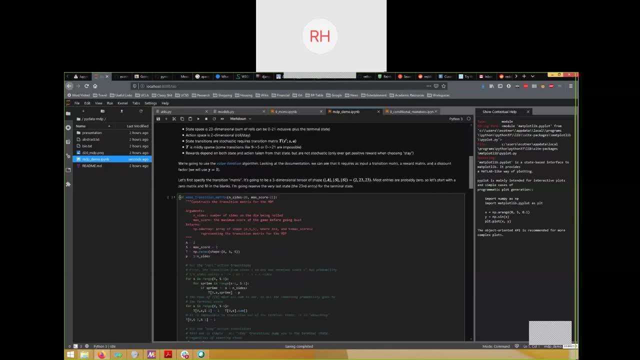 here. That's what we're using in the PyMDP toolbox for, But we're going to set up everything that you need to plug in- all the states, actions, transitions, rewards- And then you can plug that in to the PyMDP toolbox. 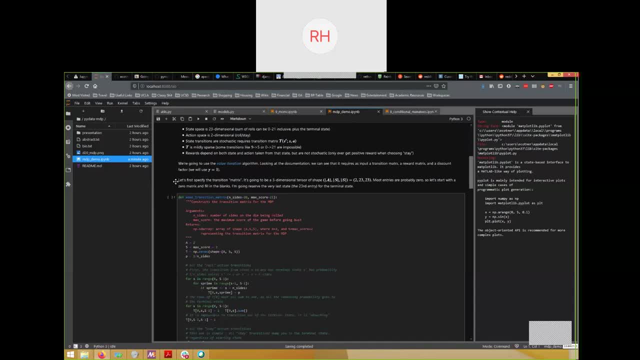 And that'll give you the stuff that you're looking for: policy and the value function. All right, so here. so we're first going to specify our transition matrix. So, like I mentioned before, in the discrete case it's generally a three-dimensional tensor. 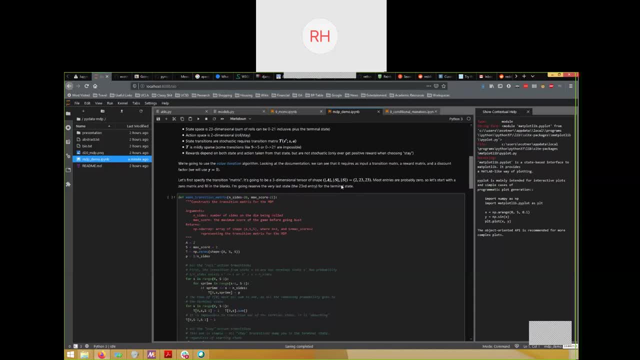 So in this case it's going to have- I remember the transition matrix maps old states, new states and actions- to the probability of those types of transitions occurring. So the, The dimension of the shape of the dimensions, is going to be 22,, 23,, 23, the same as the action state, space. 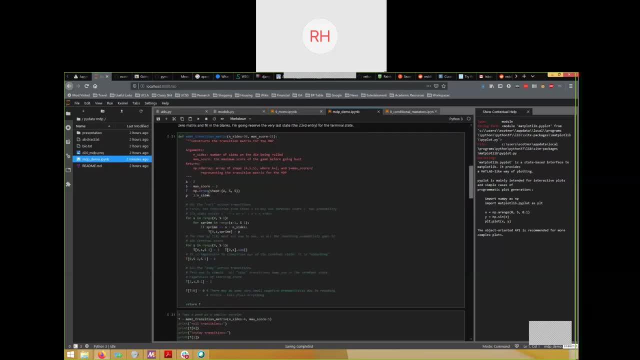 and then a bunch of zeros. So I don't know if I want to go through all of this in detail, but this is basically just me filling out all the elements. So, like right here you can see, transition from state s to any non-terminal state s has probability. 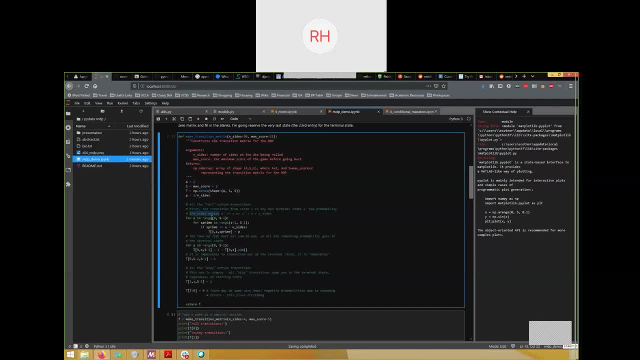 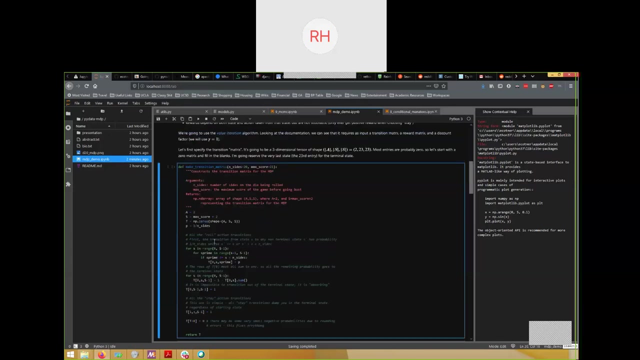 So this is going to be one over 20, because you can start at state 0 and you roll the die. you have an equal probability of ending up in any one of the states from 1 to 20.. So this just fills in those. 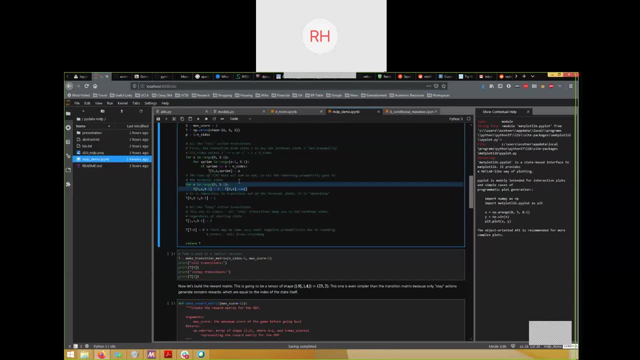 And then this one just takes advantage of the fact that the transition matrix is actually a probability distribution. So you can- You can use that to figure out what the probability of going bust is, or going to the terminal state And then the absorbing state, the final state. 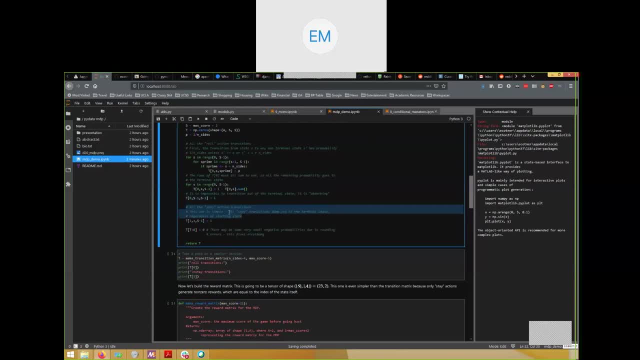 and then this takes into account all the state transitions here. So if you choose to stay, you automatically end the game. It doesn't matter what state you're in, So there's just 100% chance that you end it. And then this is just to fix any numerical rounding problems. 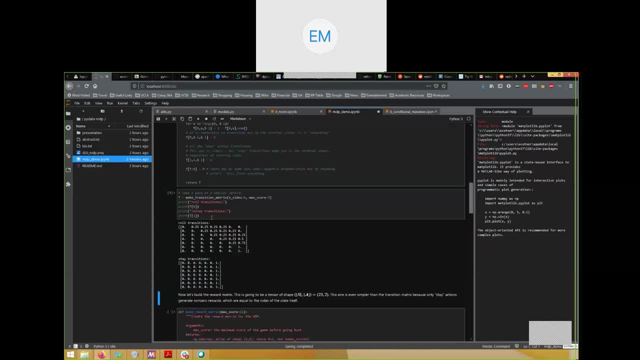 So let me run that And then, just so you can visualize it, I made the number of sides a variable, So it might be kind of overwhelming to look at all 20 at once, But this is kind of what it looks like for a four-sided die. 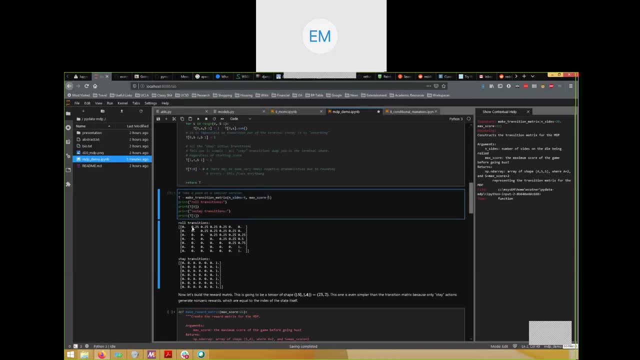 where the maximum number of score you can get before you bust is 5.. So you can see, there's zero chance that you can go from state 3 to state 1.. Wait, is that what it is? Oh yeah, that makes sense. 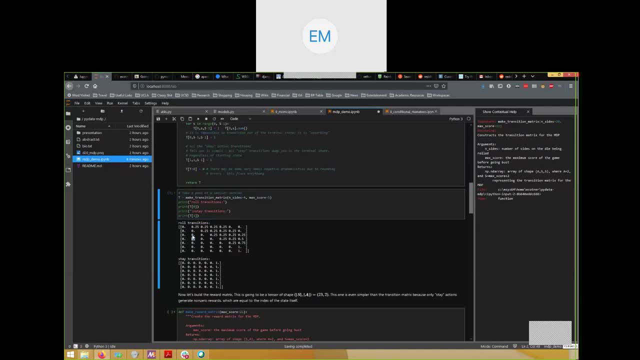 Yeah, there's no way you can go backwards from state 3 to state 1, because you can't roll negative numbers. So that's why everything over here is zeros And then everything over here is 0.25, because, since you're rolling a four-sided die, there's 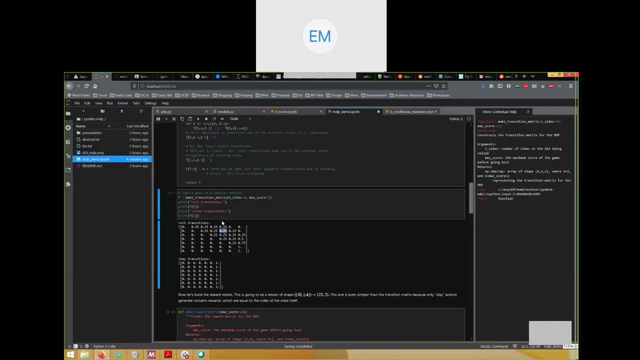 25% chance of landing on anything in the next four steps And you can also see over here in the final column. this is all the probabilities to end up in a terminal state. So as you get towards the end, it's 100% chance. 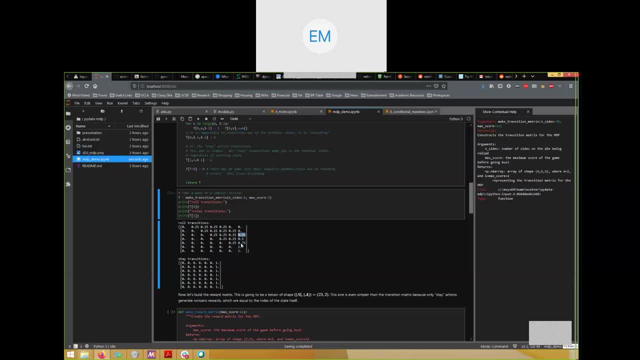 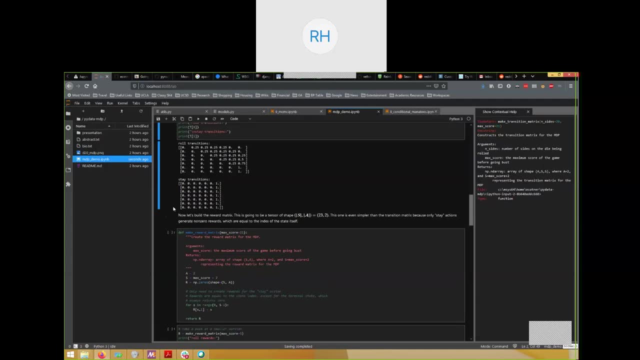 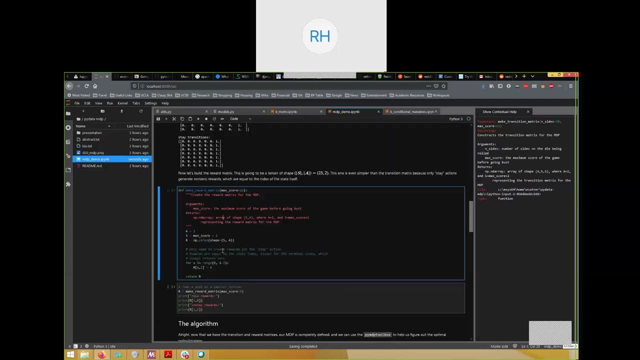 you're always going to end up in the terminal state, But the best is you have a lower number. And then the stay transition is pretty simple: Automatically end the game whenever you stay Cool. So that is the transition matrix in this case. 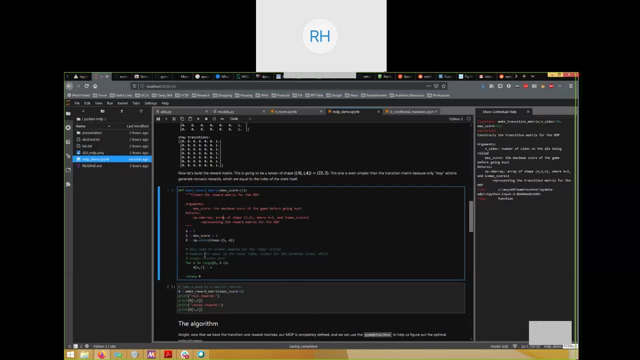 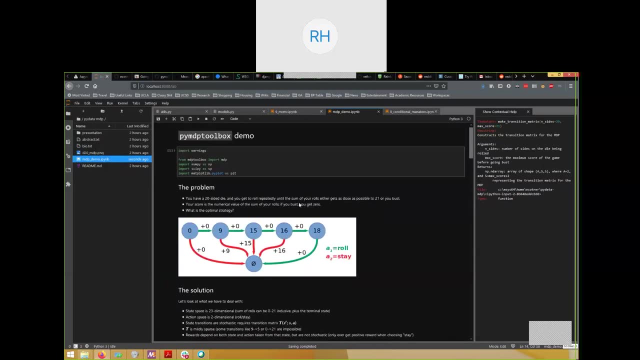 And then the reward matrix. that one's pretty simple. Oh yeah, so you only need to create rewards for the stay action, because if I go back up to my thing, you can see you don't accrue rewards by making a rolls. 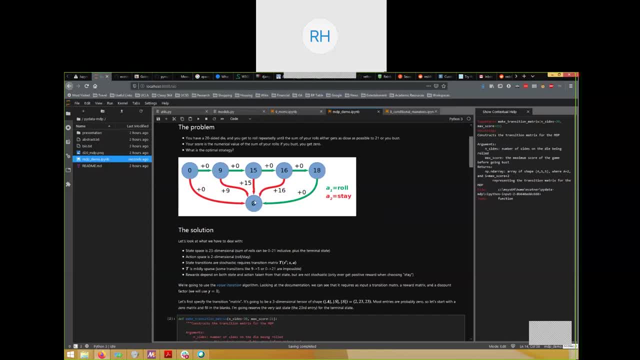 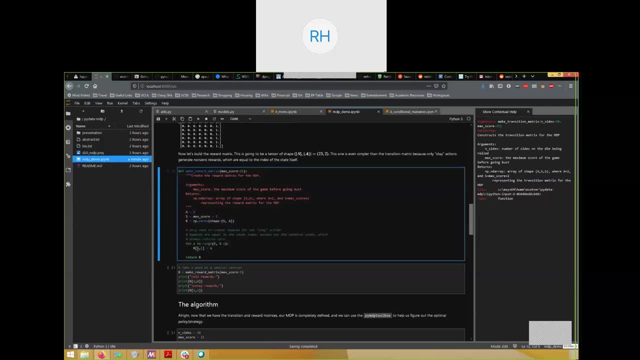 You only accrue rewards by making stay actions and ending the game, or deciding to end the game, And so the reward matrix is really simple. It's literally just whatever state you're in at the time you decide to end the game. That's how much reward you get. 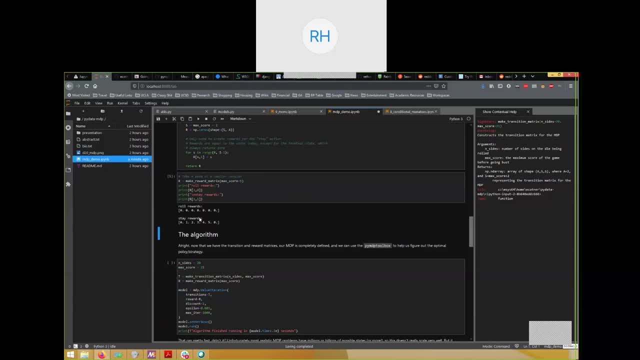 All right, so you can see for this really simple case. so if you're in state 0 and you end the game, that's really stupid of you because you get nothing. If you wait later and later, then as you accrue more points. 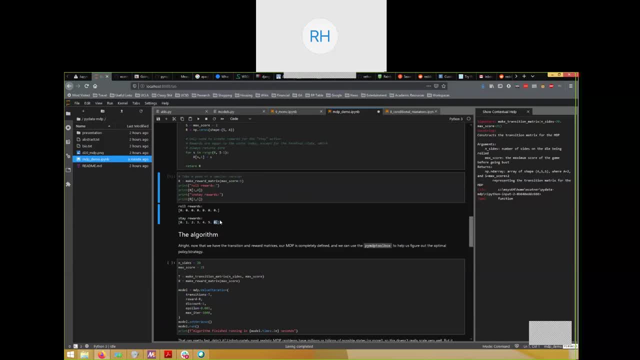 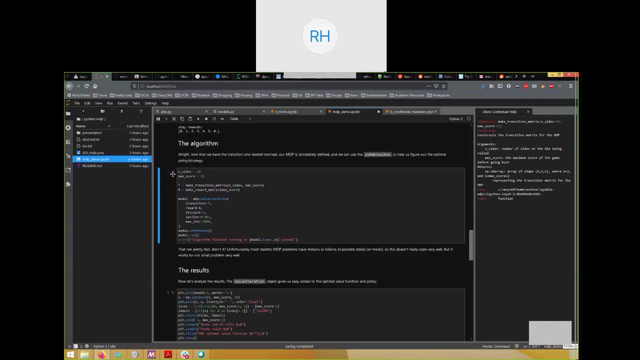 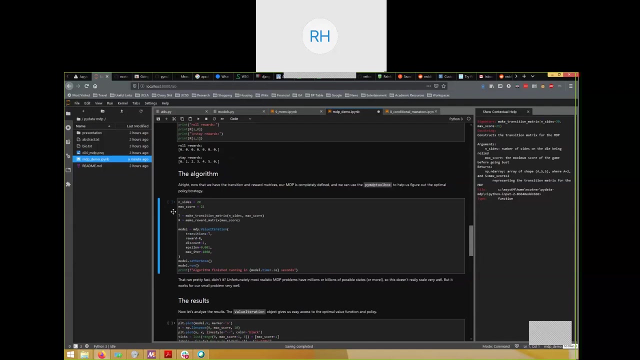 you get more reward And then the terminal state is 0, because you can't get any reward once you're in the terminal state, OK, and then finally the algorithm. This kind of covers up a whole bunch of the math, but it basically goes through the exact same policy iteration. 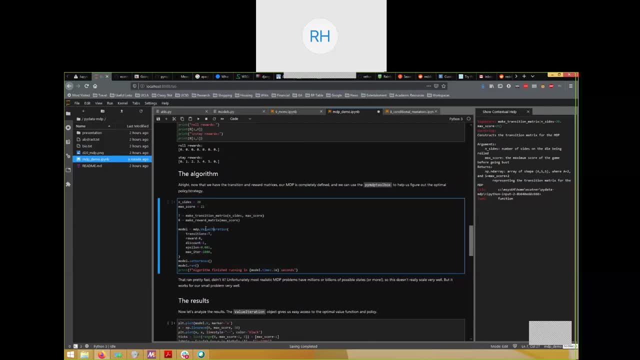 algorithm, or sorry, value iteration algorithm. See, right there, value iteration Goes through the exact same value iteration algorithm that I mentioned before. when you start off with just some totally random policy, You make it a little bit better, and then you just do that. 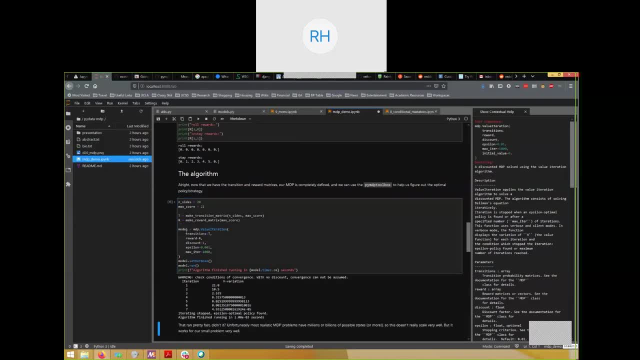 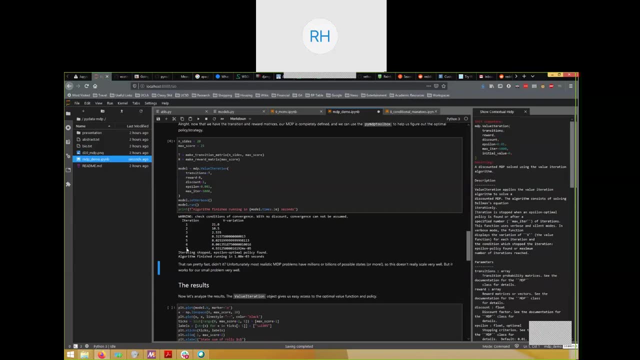 feedback loop, OK, And then you just do it until it finishes. So you'll see here that this is actually really fast because it's a pretty simple problem. So it finished after seven steps And you can see the tolerance is like five decimal places. 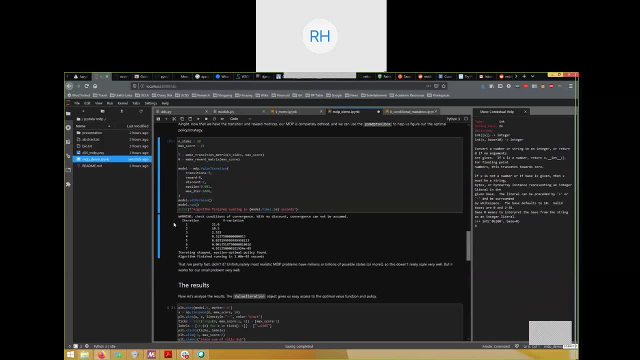 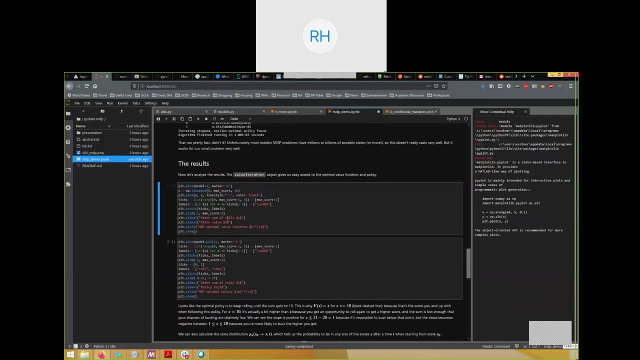 So yeah, that's it. We solved it. Congratulations everyone. So what do we do with this? now? Let's take a look. So here I'm going to plot. This is the value function. Remember there were two different value functions. 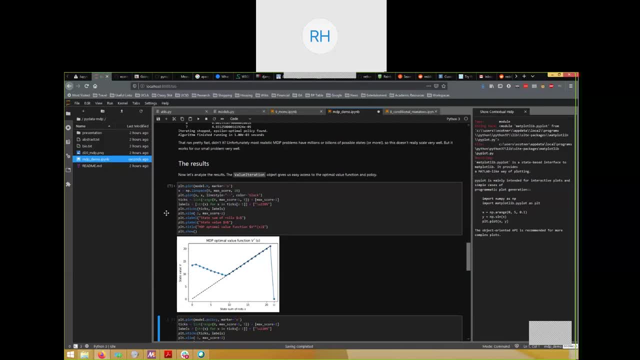 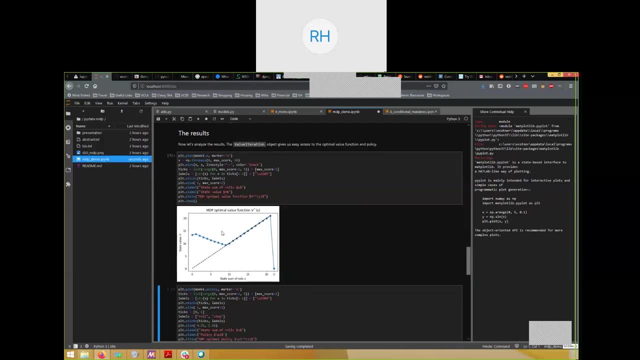 There's the Q function, which takes state and action into account, And then there's just the V value function, which is only the state, And so this is the value function for just the state value function, And you can see it looks kind of weird. 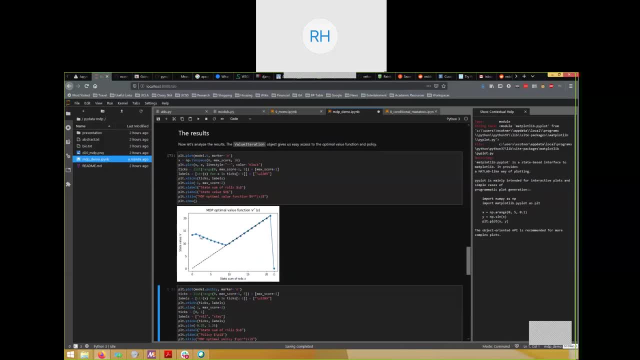 Try and do my best to explain it. I guess It starts off. Well, let's start from the right-hand side. You can see that the value of terminal state is 0, because it's literally nothing that you can do if you start off in the terminal state. 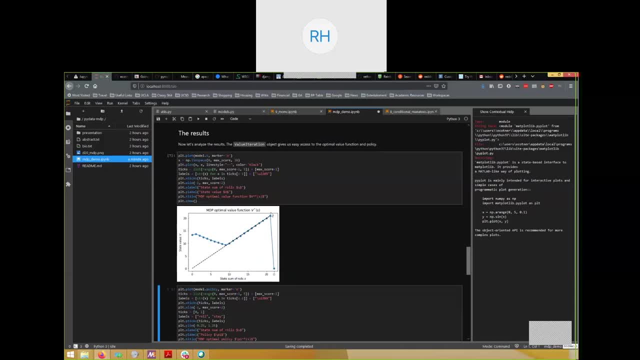 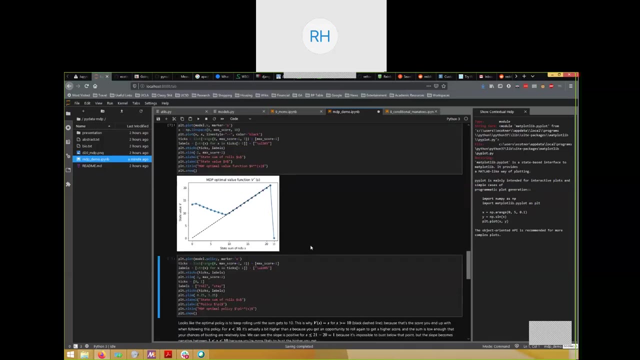 So that makes sense. And then for the right half of the states that aren't the terminal state, you can see they increase linearly with the index of the state or the sum of your rules. thus far That makes sense because once you've got the state, you're. 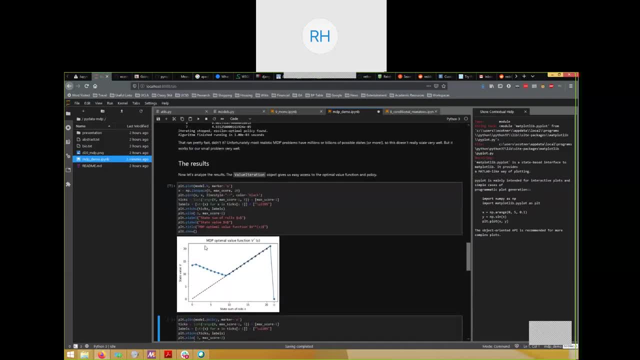 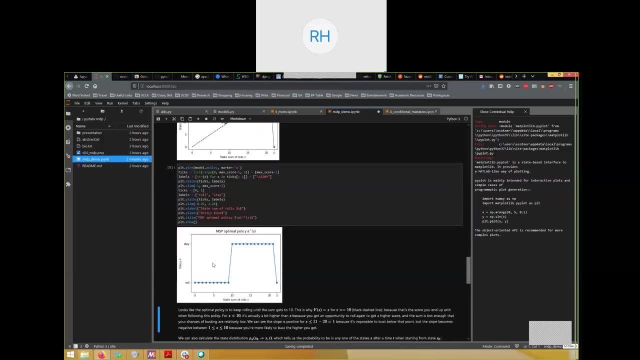 I guess it will make more sense once we look at what the policy is. But I'll give it away. Maybe it's best if I explain both of them at the same time So you can see from the optimal policy. it has decided that if you're at a sum of nine or less, 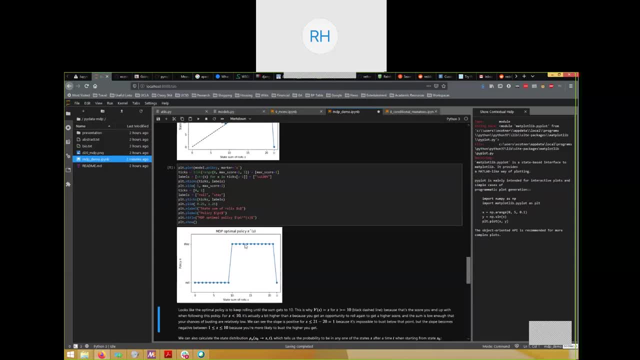 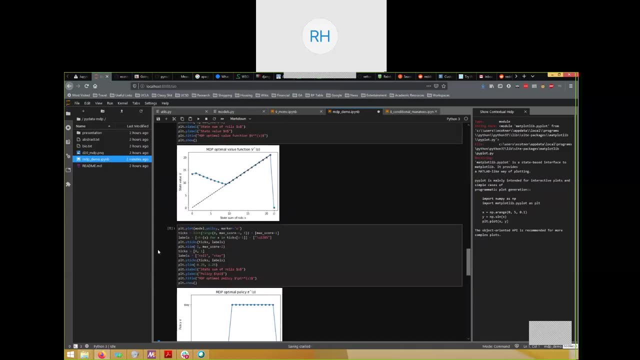 you should always roll it, But if you're at a sum of 10 or more, then you should just stop and take your winnings and go home. So now, in that context- and let me see if I can zoom out a bit- There we go. 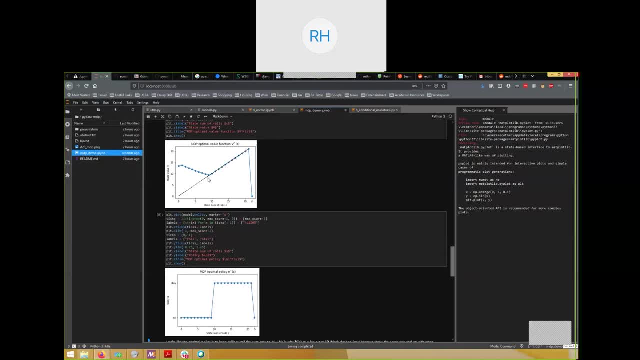 So in that context now the right-hand side of the value function should make a little more sense, because since the policy says that you should always stop, then whatever state you're in at this point, you're guaranteed to get that many points if you follow your policy. 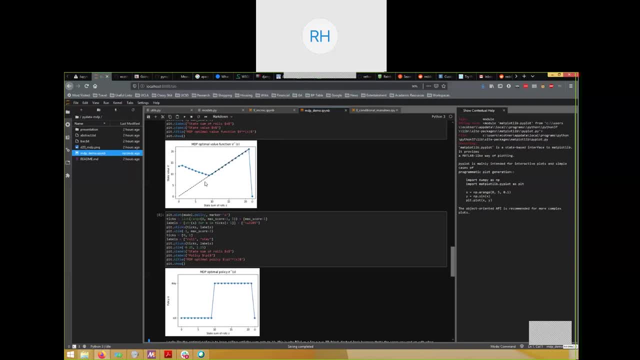 So that's why everything follows this dotted line on the right-hand side, because you get that many points by ending the game On the left-hand side. you can see there's like a little inflection And so I guess it goes downwards as your state goes downwards, as the sum of your score goes up. 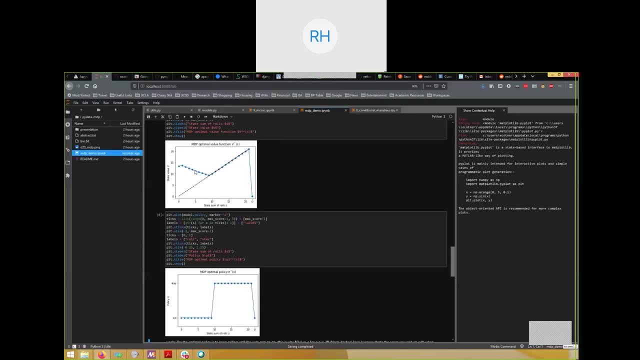 because once you get into this territory, there is now a potential that you could lose the game. Like, if you have five points and you roll, If you roll a 20, you lost. and the closer you get to nine, the higher your chances are of losing. 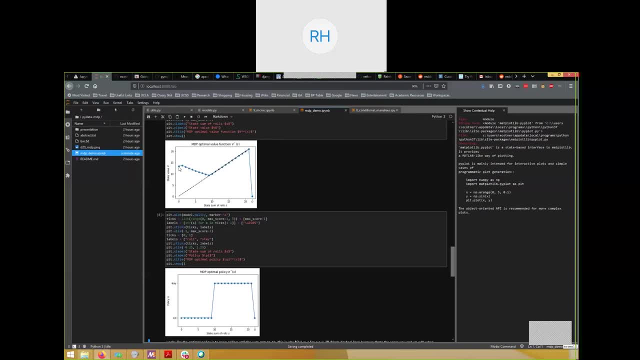 So that's why the value goes down. You can actually see on the very far left-hand side. it goes up just for one step at one, because if you're in state zero, your score is zero. there's no way that you could possibly lose. 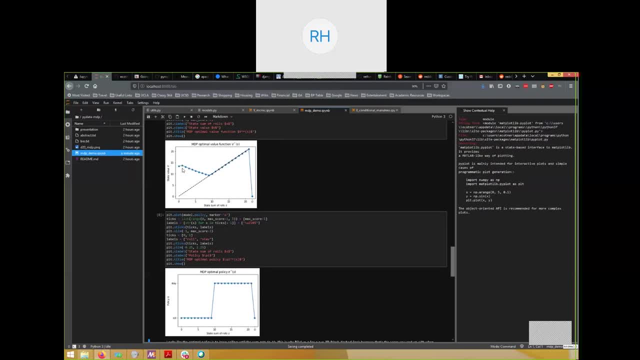 You can roll a 20, and that's great. You get a lot of points. maybe If you're in state one, there's also no way you could possibly lose. So it's always favorable to roll in that case, And if you're in state one, it's actually more favorable than being in state zero. 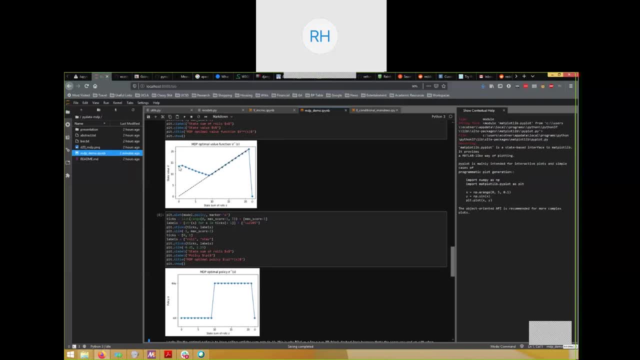 because you're always guaranteed to not lose and you're always guaranteed to make more points than if you started off in state zero. So that's why it goes up for that one step and then afterward drops, because you know You could potentially lose at that point and lose all the points that you've gained. 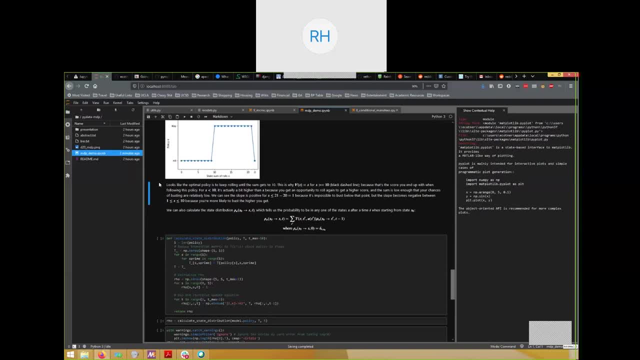 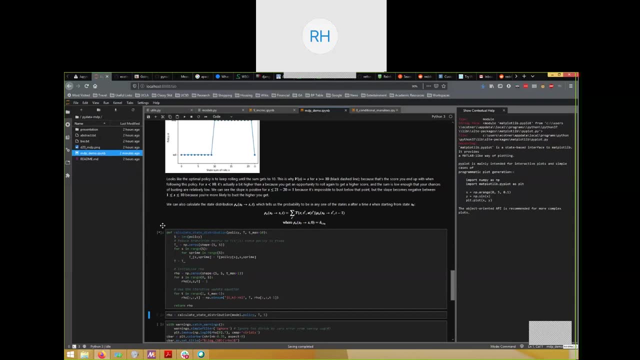 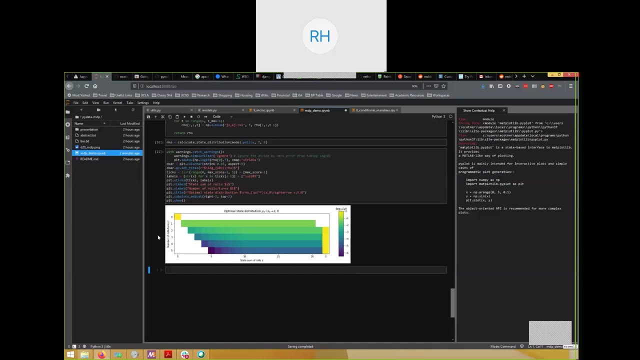 So hopefully that makes a little bit of sense. And then, finally, I didn't discuss this, but this is kind of a little extra bit So we can actually look at the state distribution, which is kind of like what is the distribution of states that you would expect to be in at any given point in time. 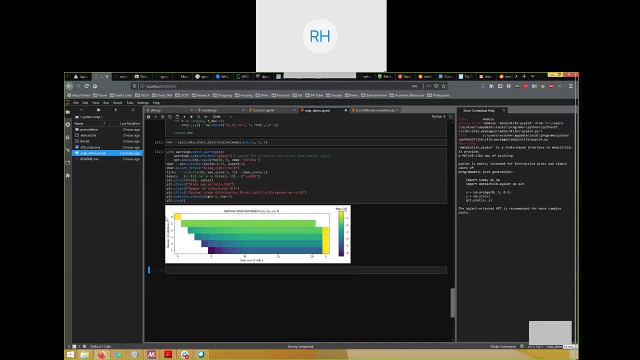 And so maybe this is potentially confusing, but time goes vertically in this plot, starting from the top and going down, So at time zero you can see all of the probability is concentrated over here in state zero, which is like you literally just started the game. so that's where you are. 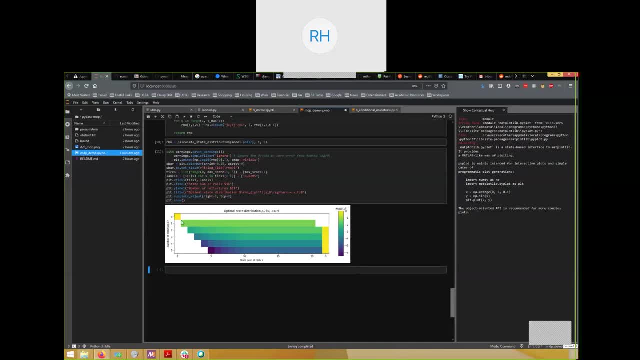 You're in state zero. But after you roll once now, there's a one out of twenty chance that all of these states over here, everything from state one up to state twenty, is populated. So this is the distribution of states that you could end up in at that point in time. 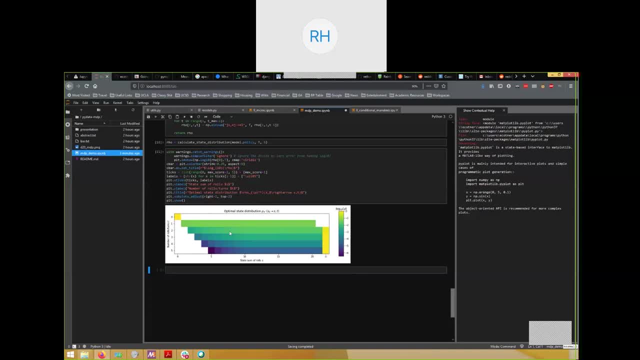 And then you roll a second time and now this is the distribution that you get. You can see now that the terminal state also has a little bit of probability of being occupied, because maybe on the first roll you got like a fifteen. You could follow that up with a ten and then you'd lose. 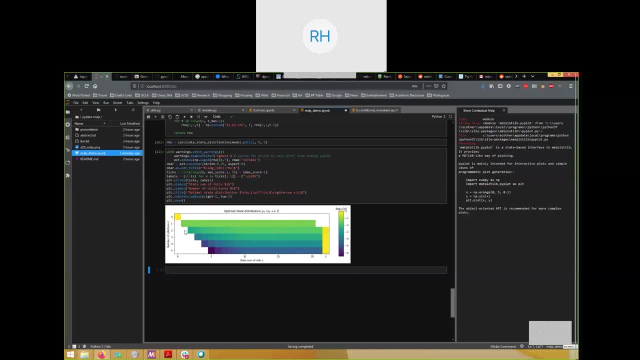 So that is potentially occupied. And then you can see that two is not occupied anymore, because there's no way that you can roll twi- Oh no, sorry. One is not occupied anymore because there's no way that you can roll twice and get one. 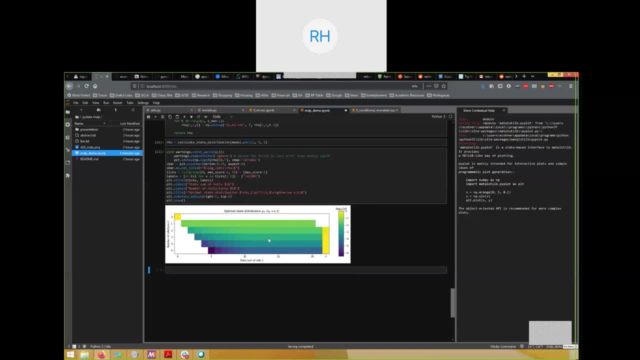 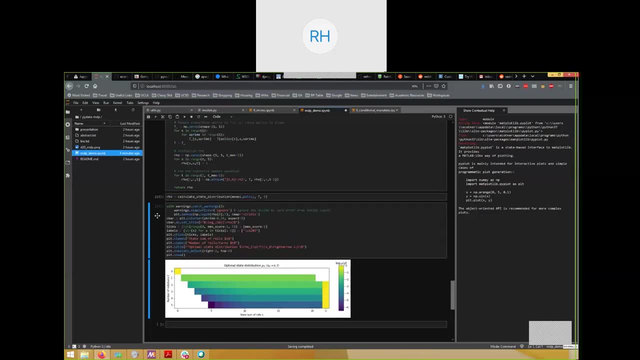 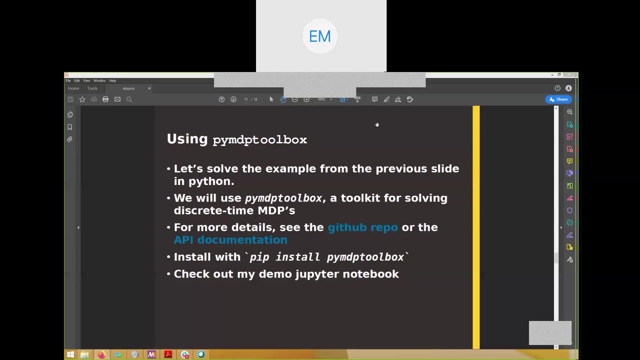 So this kind of just describes what states you could potentially be in if you follow the optimal policy. Okay, Let me go back to my presentation. Can you guys see the presentation, or is it gray now? You can see it maybe. 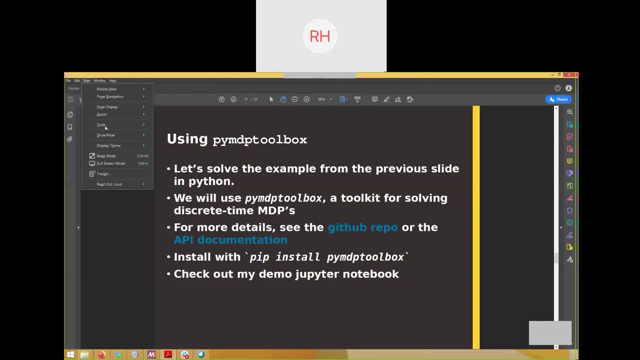 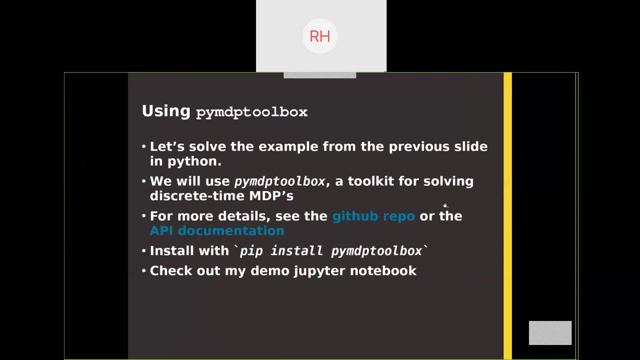 You can see it. Yeah, great, Alright, let me full screen it. Oh, full screen there, we go Cool, So yeah. so I hope you guys enjoyed that little example there And I, you know, just FYI, this is all going to be on my GitHub. 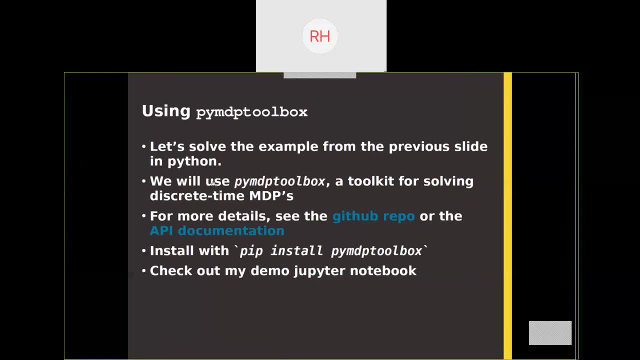 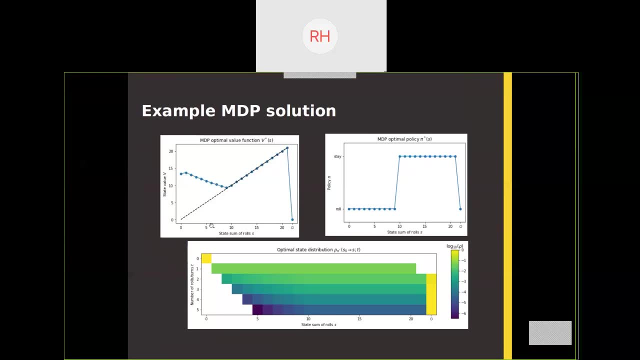 and also Pi Data, Charlotte's GitHub. so just clone the repo and go through it yourself. I guess I already explained these here, but this is the output that you get from the MDP And just to recap, summarize- you know all the stuff that we put in there. 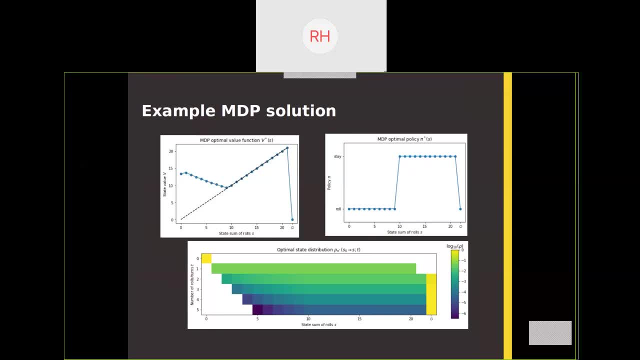 the actions, the states transitions, the reward functions. those are all inputs. And then, finally, the two outputs that we got were the value function on the left and then the policy on the right And then the state distribution. that's actually like a combination of –. 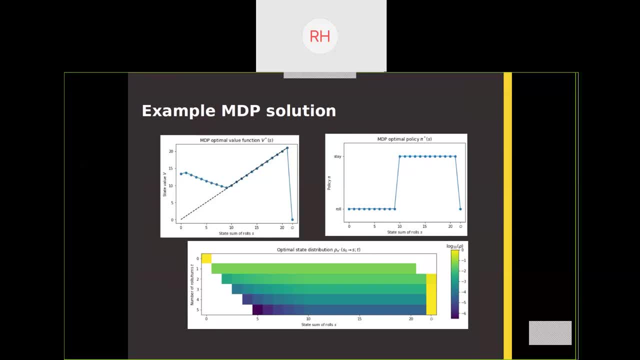 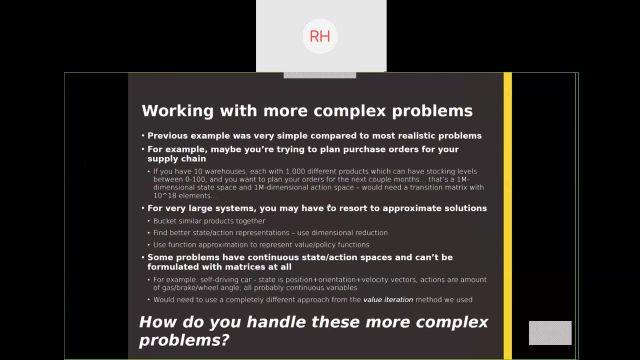 you can derive that from the policy and the transition function. So once you know the policy, then you just can automatically get that. Okay, More complex problems. So as complex as that might have seemed, problems can get like way more complicated. So the other one was pretty simple because we could actually enumerate every single state. 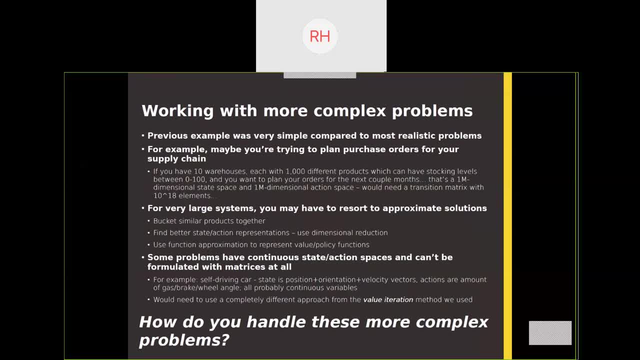 But in like a realistic scenario where you want to do this to optimize something in a supply chain, for example the – we run into the curse of dimensionality where the transition matrix that we discussed, because it has two dimensions for the state space. 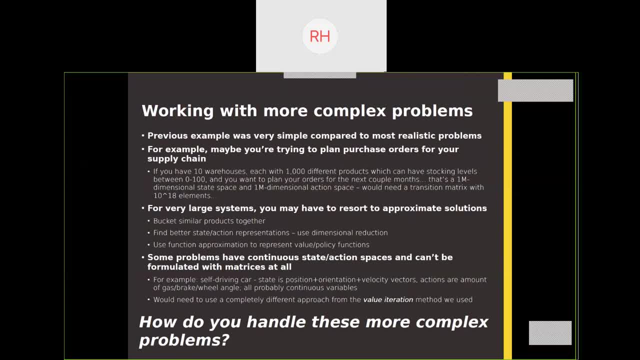 There's like the old state and the new state plus the action space. It's just like a huge explosion of elements in that matrix. I'll just give like an example here: If you have 10 warehouses, 1,000 different types of products, 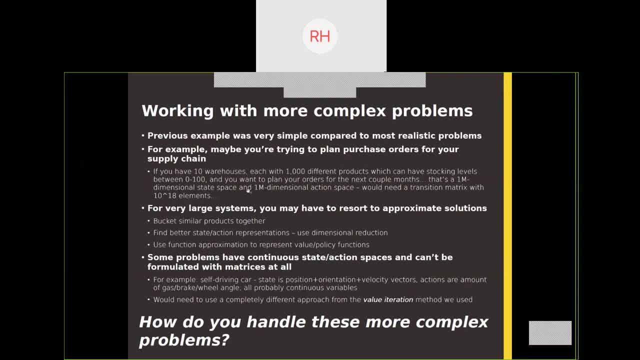 they all have stocking levels between 0 and 100.. Now you want to plan your orders for the next couple of months. Well, your state space is – like. if you say your state space is like I have this much product at – sorry, I have this much of this type of product at this warehouse. 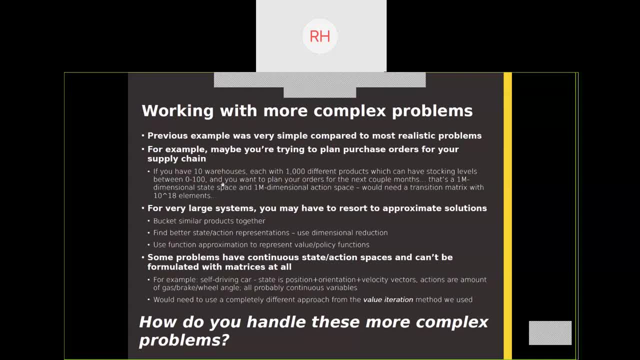 that's a million-dimensional state space. You just multiply 10 by 1,000, by 100.. And then – so your transition matrix – oh, and then also a million-dimensional action space, because you need to say how much of that product you're moving to this warehouse. 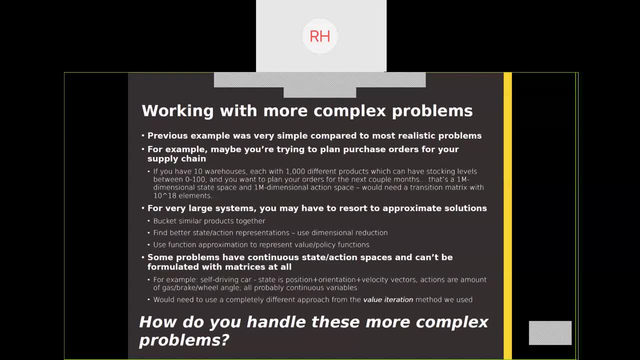 You get 10 to the 18 elements in your matrix, which is just ginormous. There's no way that you could feasibly compute anything with that. So for systems like this, you have to resort to like approximate solutions, And this is –. 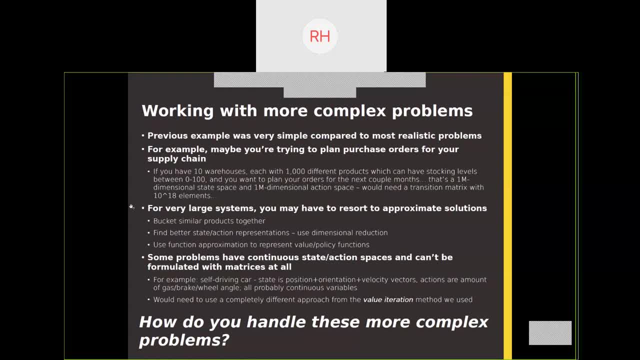 this is more of an art than a science. There's a lot of tricks you could do If you want to try and you know, can bucket all the products together, like maybe some products are, like, really similar to each other, Like if you're selling umbrellas. 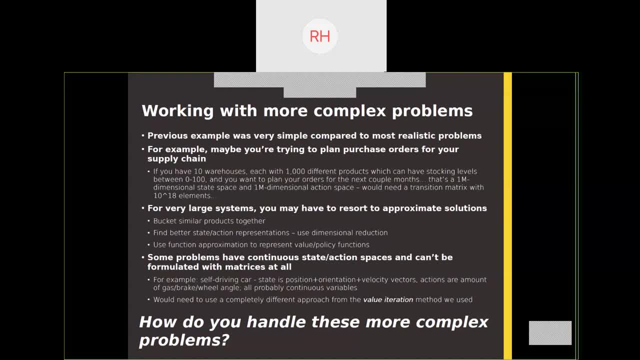 you can bucket different colors of umbrellas together because maybe people don't really care that much. You could try and get better state and action representations, So like in the very very first example that I had, if you're rolling the die and you know, 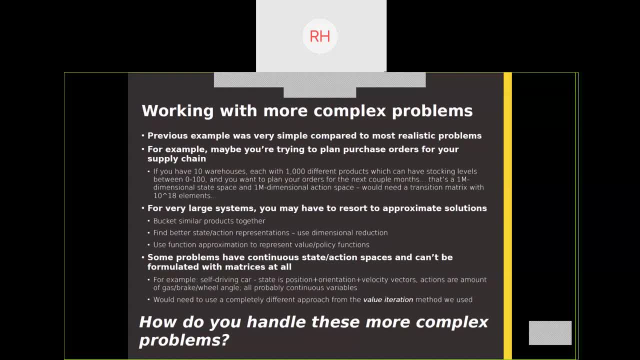 two sides lose you money and four sides win you money. I had two different state representations. There was the one representation where every different side was its own state, but then there was also another representation which was like those two sides were the same state. 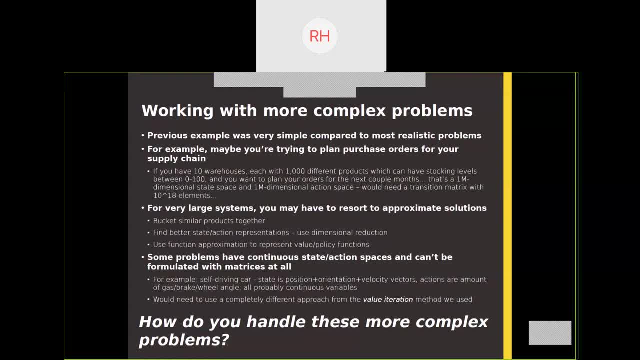 because they had the same payout and then the other four sides were technically also the same state. So you can use tricks like that to try and make your state space smaller, like easier to compute. And then, finally, you can use function approximation to represent the function. 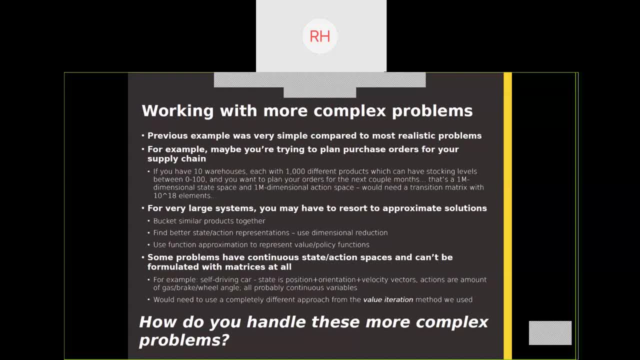 So this would be something like using neural network, for example, or linear regression. rather than using a matrix to explicitly model every single transition, probability and whatnot, You can use some sort of continuous function that's parameterized by learnable parameters. So that would be another way of tackling it. 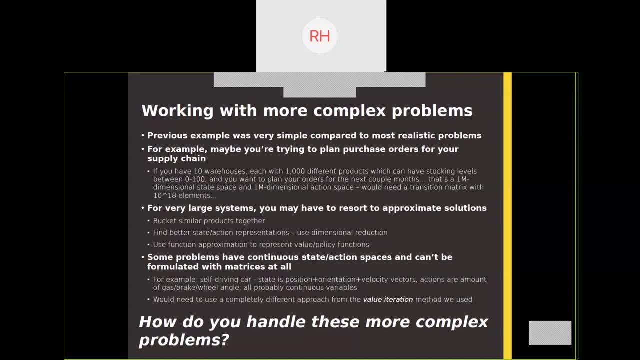 The other complication, which I think I might have touched on a bit previously, was the other thing we talked about up to now was discrete action spaces and discrete state spaces, but you could have continuous spaces as well, So they'd literally be like an infinite number. 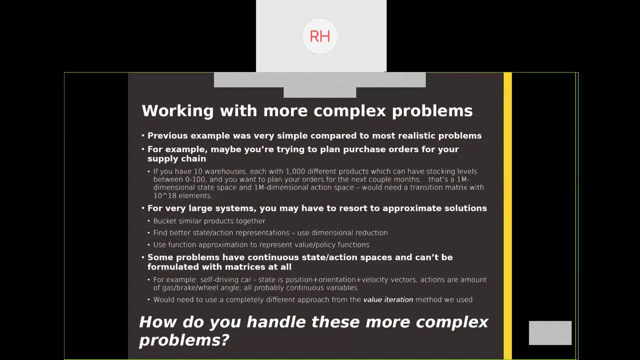 an uncountably infinite number of states and actions, And the the self-driving car was, I think, an example I mentioned earlier. You know you could have different, continuous variables for the angle of the wheel, for the angle, the amount of pressure that you apply to the brake. 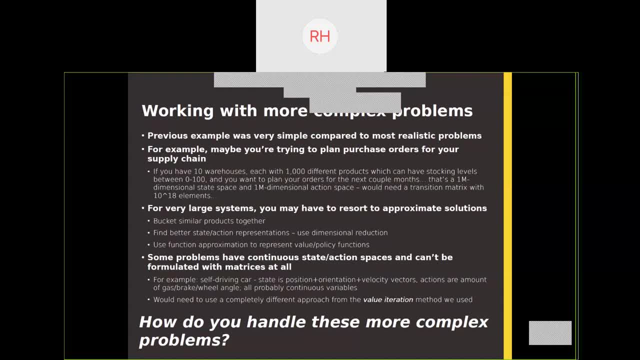 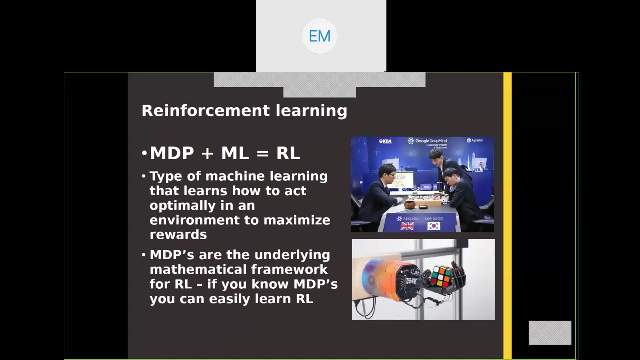 stuff like that. So those, those can all be continuous, And in this case the value iteration completely fails. There's no way you can handle. you can handle continuous variables, So so how do you handle these? Well, reinforcement learning is typically the next thing that people have reached. 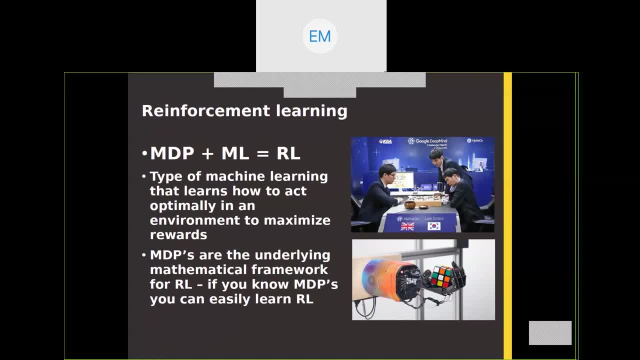 for because it combines machine learning and Markov decision processes So you're able to learn from like very high dimensional data sets. Like the picture on the right you can see, this is the, the AlphaGo algorithm, which beat the world champion at. 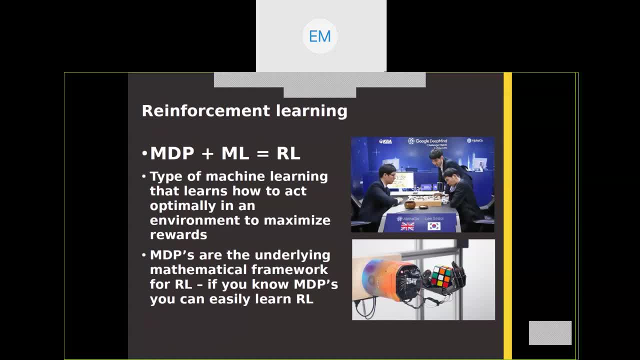 at Go The states, the state space in Go like, if you try, and you know, enumerate every single possible layout of the board is just like astronomically high. I don't know the exact number, So there's no way that you could build a transition matrix for every single element there. 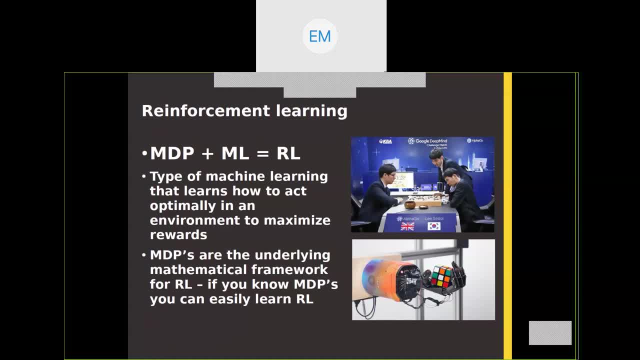 You have to use some sort of function approximation And machine learning is like very, very good at learning patterns in these very high dimensional states, So that's usually the thing that people, people turn to, And there's a lot of like super, way more complicated algorithms that you can use. 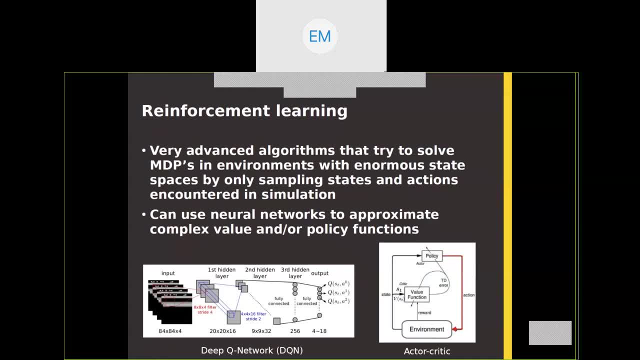 as opposed to value iteration. Value iteration is literally like the simplest possible thing There's. there's all sorts of crazy things I wouldn't like. a really common one is the deep queue network which you may have heard of, but it's. 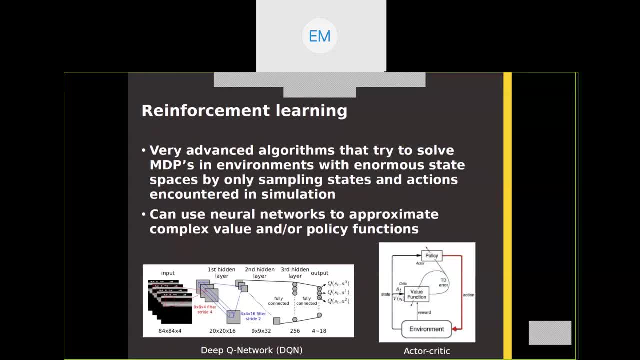 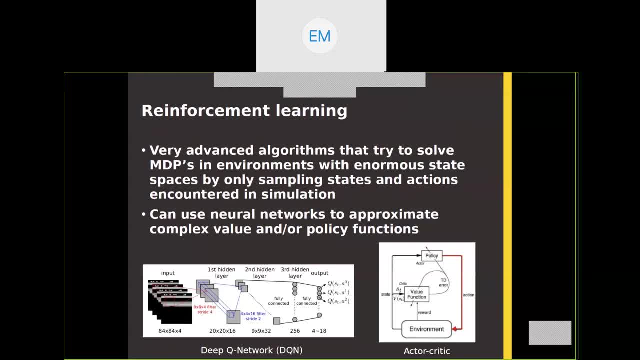 it's it's it's specific to Atari games. So the the queue network works in cases where your state space might be continuous when your action space is discreet. So it works really well for Atari where you have like you're a joystick where you like. 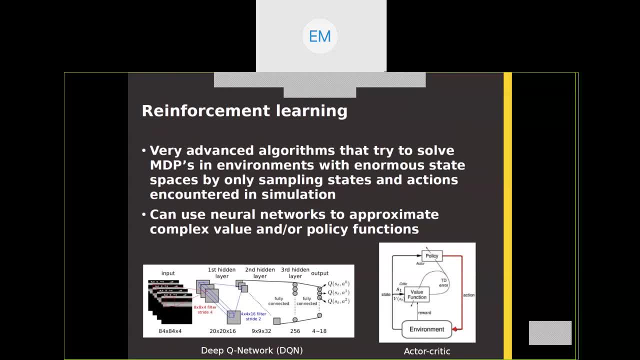 move left, move right, move up, press A and B buttons, stuff like that. There are also other algorithms like DDPG, DNS, deep deterministic policy gradients- Any algorithm you hear of that has the word policy gradient in it. that means that it works in continuous action spaces. 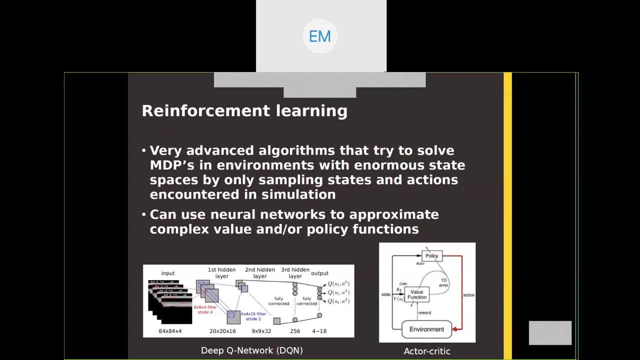 because you're kind of taking the gradient of the action space that shows up in the updated version. Oh, and you can see on the bottom right actor critic. That's kind of like another flavor. Actually it's like a combination of the Q learning. 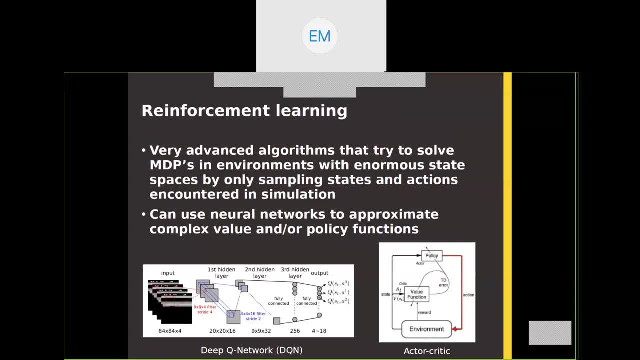 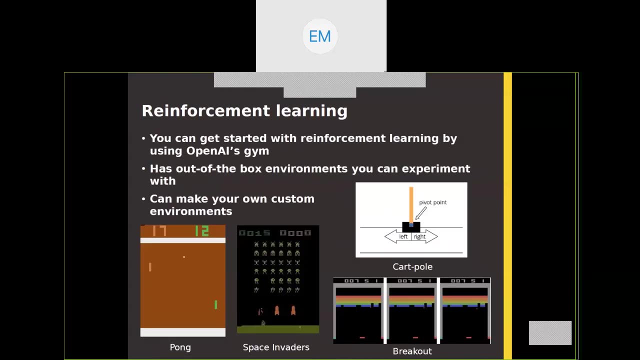 the Q network and the policy gradients. So there's like a whole plethora of different types of algorithms that you can use, And almost all of them work with neural networks. That's like where all the cutting edge research is done in this case. 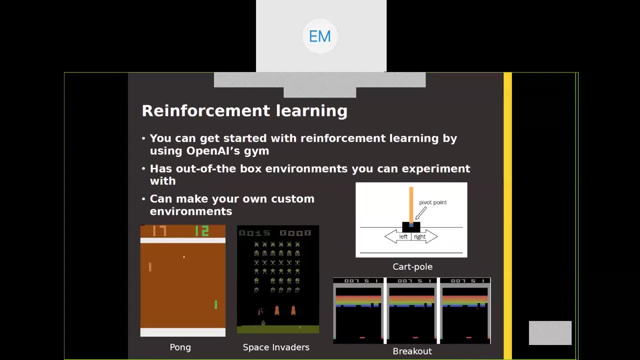 Oh yeah, here you can see the Atari examples. I also want to point out: if you want to get started with reinforcement learning and MDPs and whatnot, you should go To OpenAI's website. they're the company that did the OpenAI 5, which it was like an AI that could play. 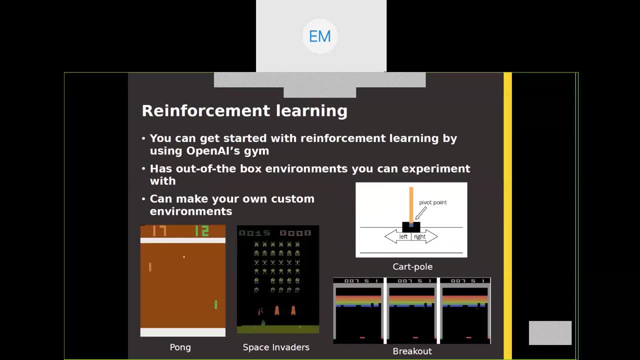 Was it Dota, I think. Was it League of Legends, I don't remember. It was either Dota or League of Legends. Yeah, it's Dota, Dota, OK, yeah, So they taught some reinforcement learning. They taught reinforcement learning agents.